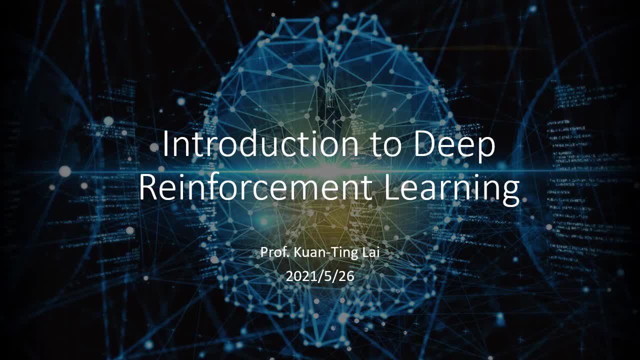 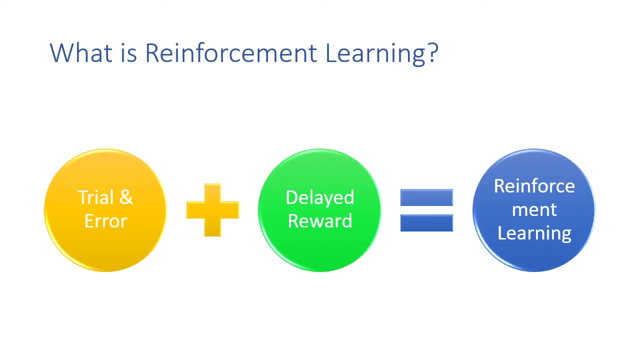 Hello, everyone, welcome to join us. Today we are going to talk about the deep reinforcement learning the theory behind ABAGO, the program that beat human goal champion. Deep reinforcement learning is one of the most exciting research field in recent years. What is reinforcement learning In its simplest form? 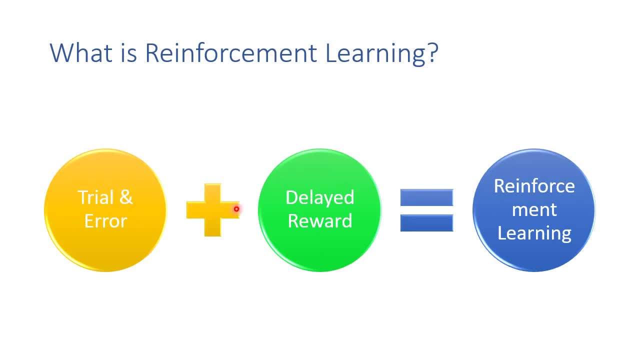 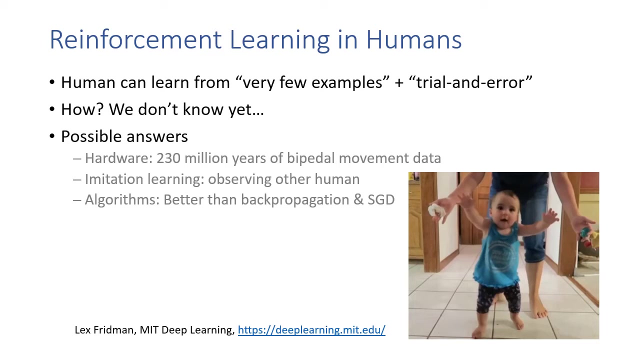 reinforcement learning is trial and error plus delayed reward. Trial and error means learn from your own mistakes, while delayed reward means our goal of learning is to maximize the cumulative reward in the end. In fact, there are a lot of reinforcement learning, examples of animals, For example. 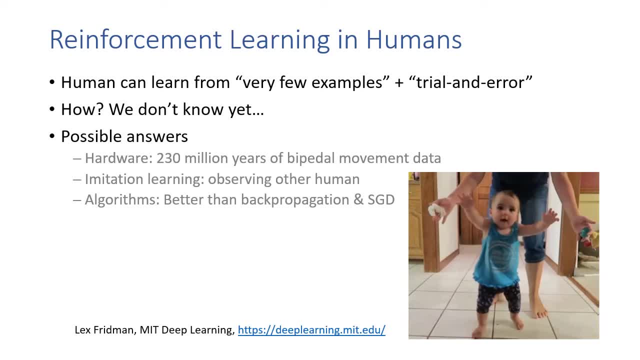 let's think about a baby. Let's say it's a very tiny baby. It's a child that tries to learn how to walk by myself. They will keep falling and standing up, falling and standing up many, many times until they learn how to walk. However, there is a big difference between today's reinforcement learning algorithms. 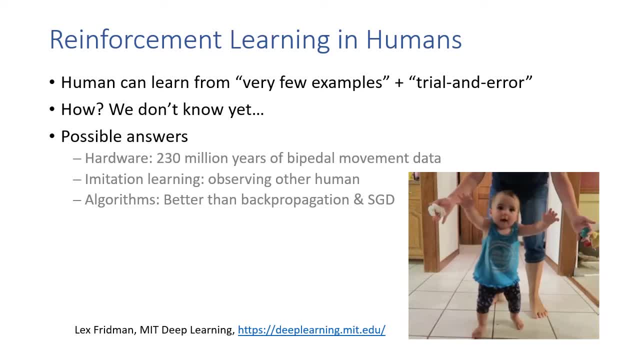 and the animals' learning, that is, animal and human can learn from very few examples. This is an unsolved problem and we still need it. Thank you for watching. If you like the content, please share the video and leave a like. It will be appreciated. See you in the next video. Bye. 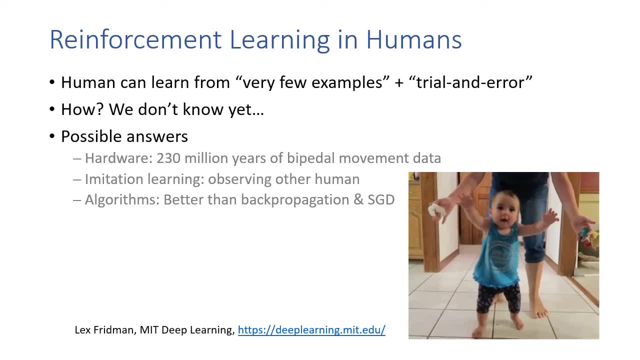 don't know why. The possible answers are: maybe that animals have some pre-programmed algorithms in their brain after the 230 million evolution, or humans can do imitation learning by observing other humans, or that we need better algorithms that current backpropagation and gradient descent. 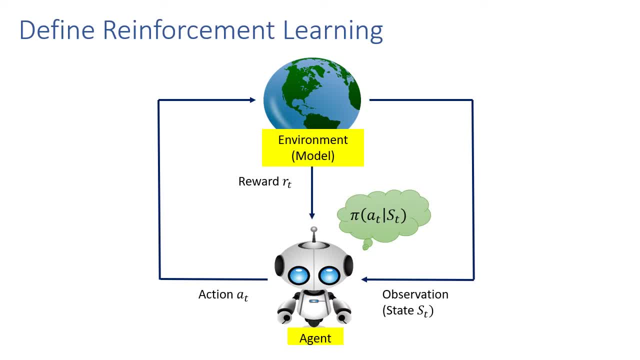 Let's define reinforcement learning mathematically. First, there is a software agent and an environment. The environment provides observations and rewards to the agent. Observations is also called state. The goal of the agent is to learning how to perform different actions under different state. 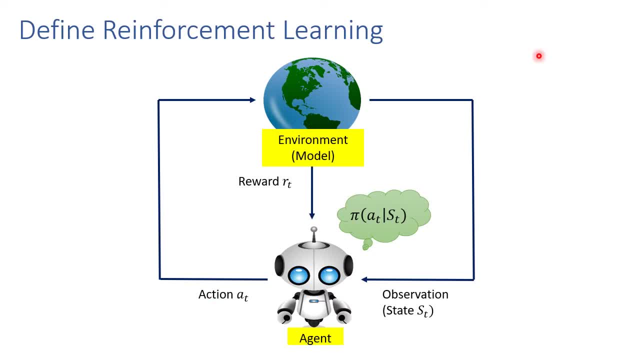 In order to achieve maxima cumulative future reward in the future. In other words, the software agents learn and optimize action model in an environment by doing trial and errors million times. The model is also called policy. We can use conditional probability to represent policy, So policy can give us the 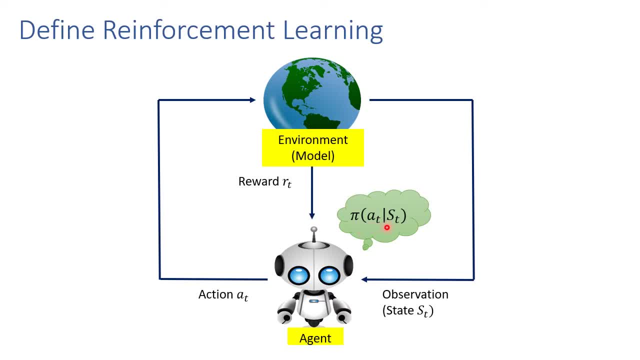 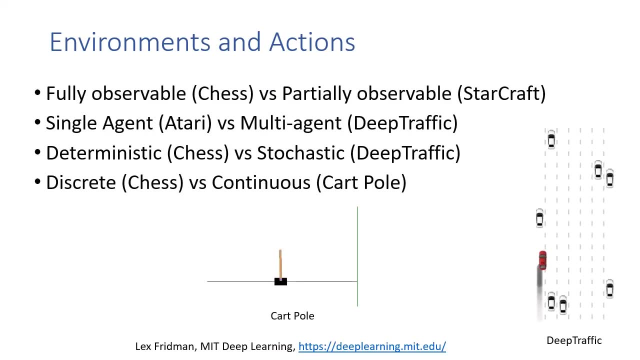 probability of perform action under the observation. There are many kinds of environments and actions. as listed in this slide. Chess is fully observable, which means that we can observe all the actions of our opponents. On the contrary, the video game Starcraft is only partially observable. 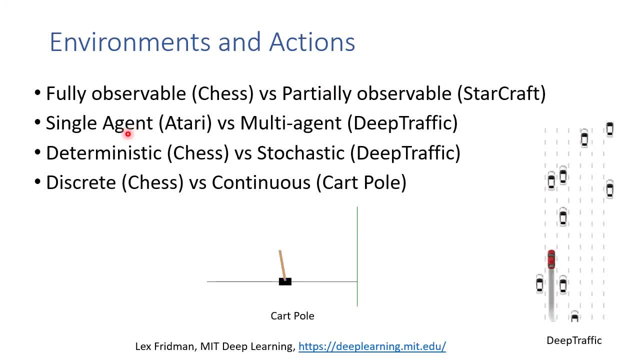 The other characteristic is if the learning is performed by single agent or collaborative learning of multiple agents. The simulation environment developed by MIT professor Lex Friedman- By the way, many slides are extracted from his lecture- Deep traffic. The simulation environment deep traffic, developed by. 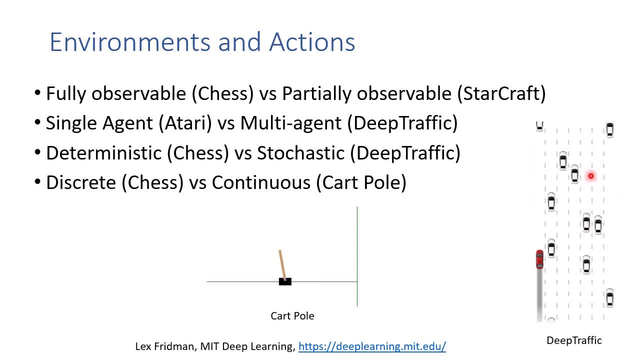 MIT is an example of multi-agent. The simulation environment deep traffic developed by MIT is an example of multi-agent Learning, which is shown here. Another characteristic is whether the environment is deterministic, like chess, or stochastic, which has some randomness in the environment, like deep traffic. 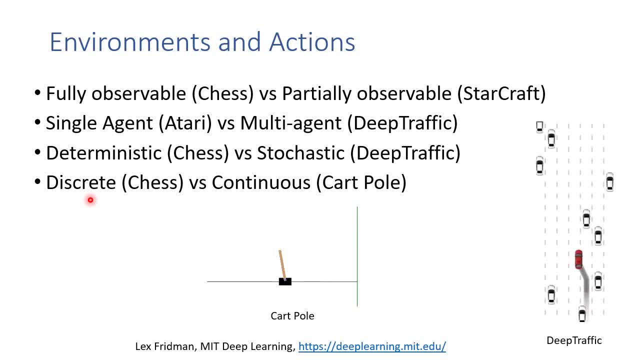 Finally, the environment can be either discrete or continuous. Reinforcement learning can be formulated as Markov-Delta environment. gera potential którą mibility cwc vai trовор pase trblowing. Reinforcement learning can be formulated as Markov-Delta environment. Reinforcement learning can be formulated as Markov-Delta environment. Reinforcement learning can be formulated as Markov-Delta environment. Something else that will hurt students: An Girls Day s3 spoon nest is to comprise courses with game learning on billion dog technology. resentment top in another place in a story that is looping in a group and sell to fans over 100 children by using brain cells. In addition, temperament, Josh O делать has a special research called performance. does the reading atmosphere? clearly performing no particular needs. 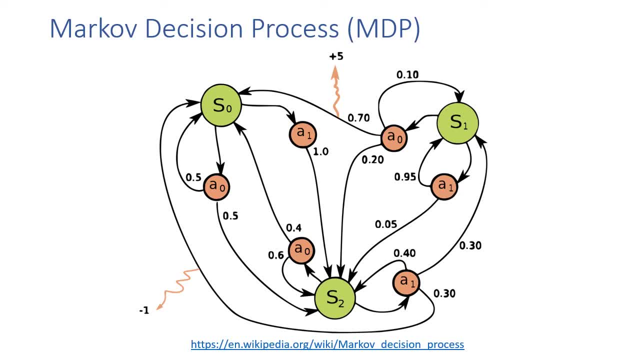 as Markov Decision Process, which is a discrete-time stochastic control process. Here is a figure of NDP process, which extract from the Wikipedia. NDP has widely used in many disciplines, including robotics, automatic control, economics and manufacturing. NDP were proposed as early as 1950s and provides a mathematical framework for modeling decision-making in situations where outcomes are partly random and partly under control of a decision-maker. 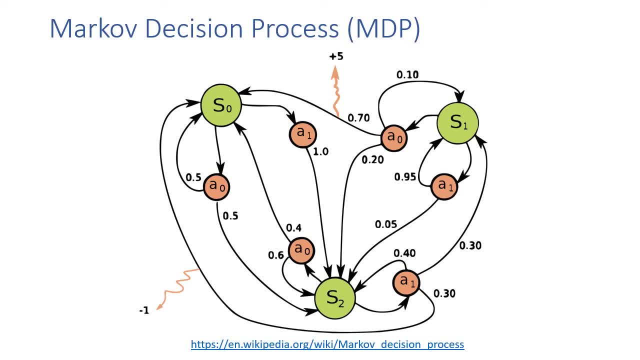 NDP are useful for studying optimization problems solved via dynamic programming and reinforcement learning In this figure at each time step. the process is in some state S and the decision-maker may choose any action- A0 or A1 in this case- may choose any action that is available in state S. 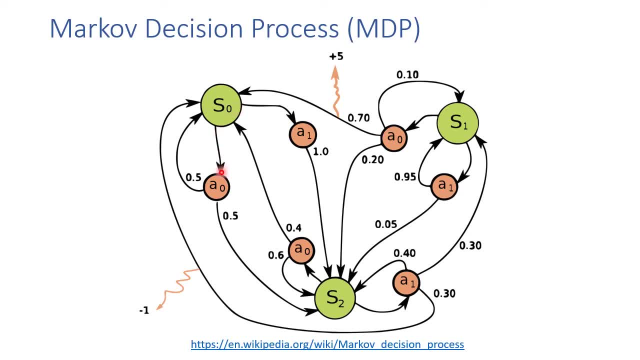 Once you choose an action- suppose it's A0, you have a randomly. you may be randomly moving into new state. In this case, we have 0.. 0.5% probability to move to state to go back to state 0, or 0.5 probability to go to state S2.. 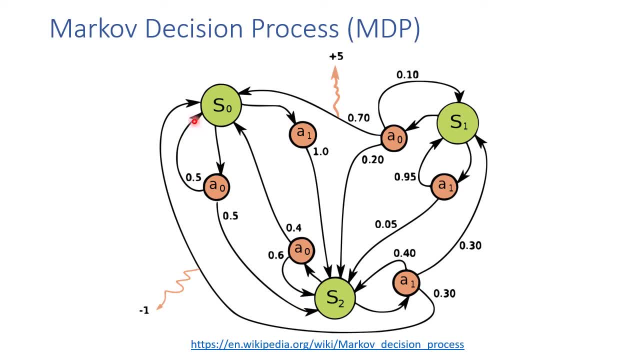 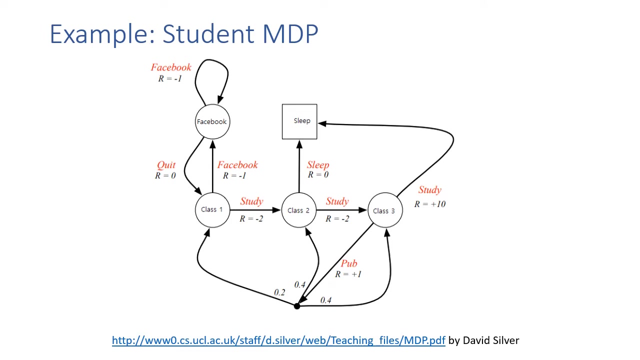 Each action, each random result will give us a reward. Here this is minus 1 reward. here is plus 5 reward. So this is this process is partly random and partly under control. This is Markov Decision Process. Here is an example from David Silver's class. 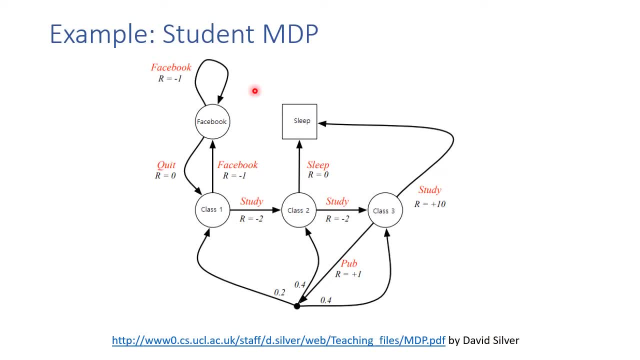 He created a student NDP Markov Decision Process example. In this example a student first go to class 1.. After the first class, the student may choose to do Facebook or continue to join the next class, Class 2.. If you can insist to go to class 3 and continue studying. 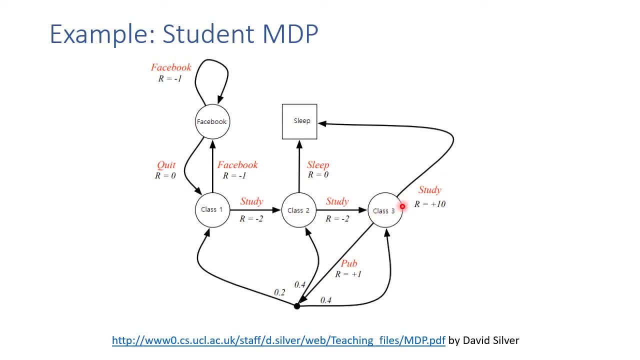 then you will pass the class and get the reward: class 10.. And then go to the final state, the terminal state, SLEEP. SLEEP is the terminal state of the student NDP, So once we reach terminal state, we will stop here. 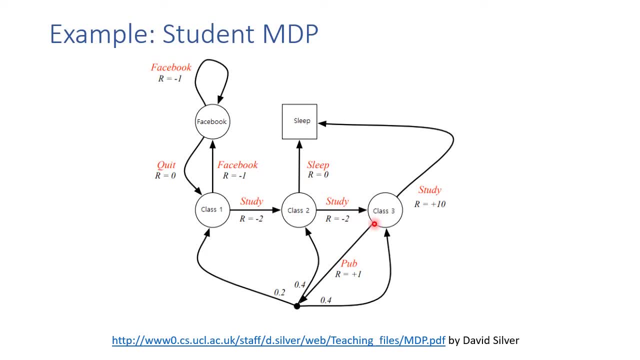 On the other hand, after class 3, you may choose to go to pub and relax. Then, after the pub, you will randomly go back to review the material. Maybe you have a discussion with your friends So you may decide to. you have 20% probability to decide to go back to review the material of class 1.. 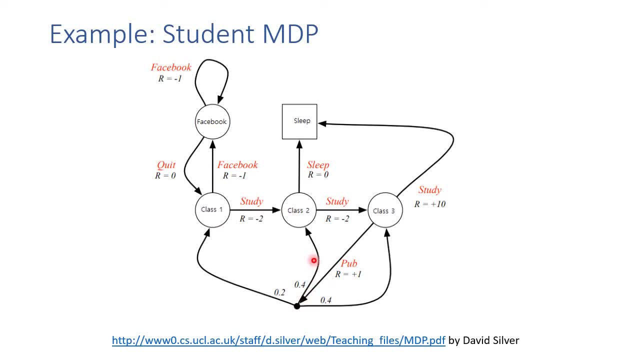 Or 0.4 probability. Or 0.4 probability to go to review class 2.. Or 0.4 to go to class 3 and continue to study the material of class 3.. And finally, you may again choose to pass the class and get the final reward: class 10.. 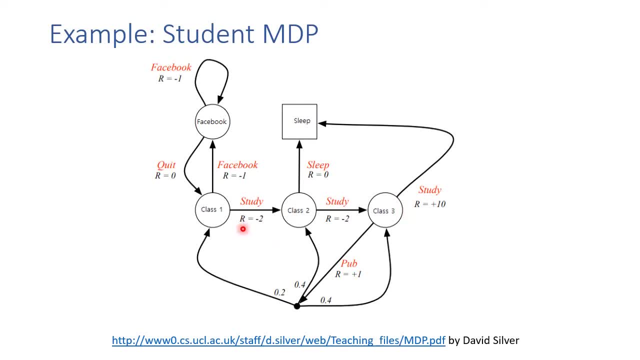 We may notice that there are many minus rewards. It's very natural. It's reinforcement learning. For example, doing Facebook will hurt your learning, So you get minus 1 reward. But, however, study may also hurt your feeling, So you may get minus 2 reward. 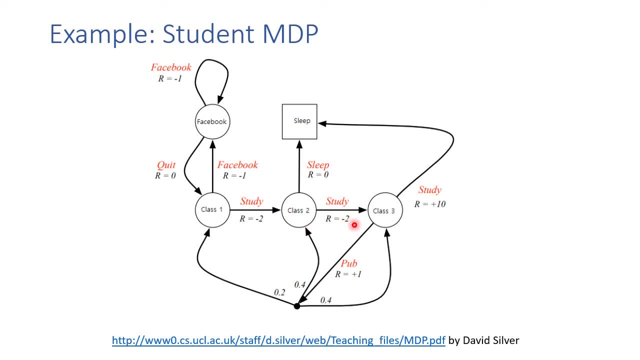 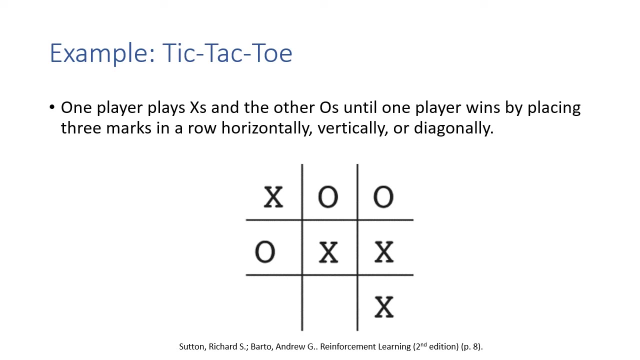 After the first two classes. that's very similar to real life. Study is painful, but you will finally get your reward in the end. Let's look at another type of reinforcement learning which is related to chess game. Consider the familiar child's game of tic-tac-toe. 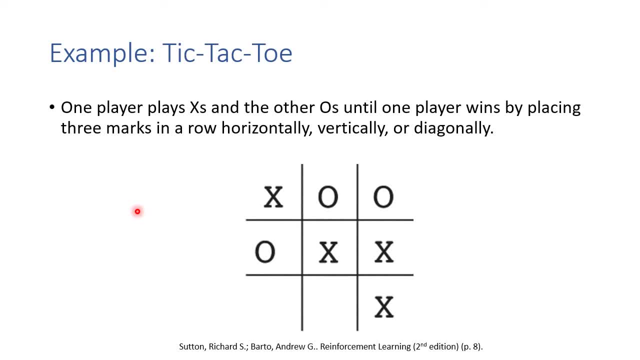 Two players take turns playing on a 3x3 board. One player play X and the other play O, Until one player wins by placing three marks in a row: horizontally, vertically or diagonally. As shown in this figure, the X player has won because it plays 3x diagonally. 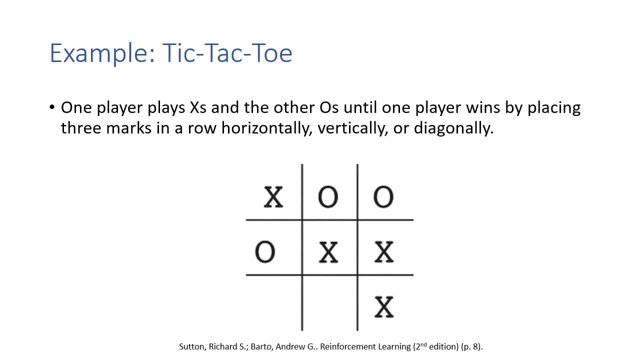 If the board fills up with neither players getting three in a row, then the game is a draw, Because a skilled player can never lose. let us assume that we are playing against an imperfect player, one whose play is sometimes incorrect and allows us to lose. 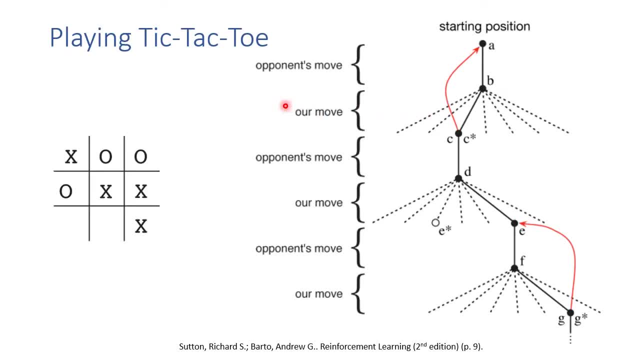 Then the game is a draw. When playing the game, our move will affect the opponent's move and the opponent's move will affect our move. This process can be expanded into a tree structure. If the number of sets is small, we can exhaustively calculate all the winning probabilities. 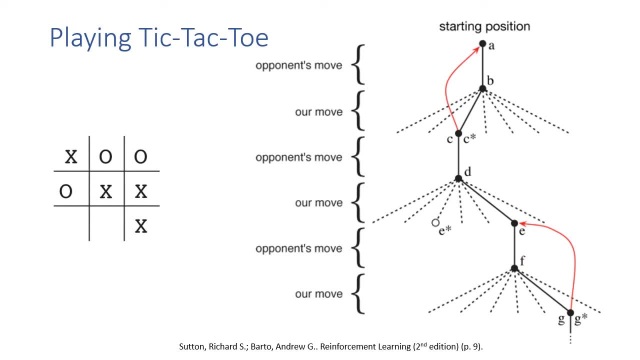 First we will set up a table of numbers, one for each possible state of the game. Each number will be the latest estimate of the probability of our winning from the state. We treat this estimation as the state's value And the whole table is learned. 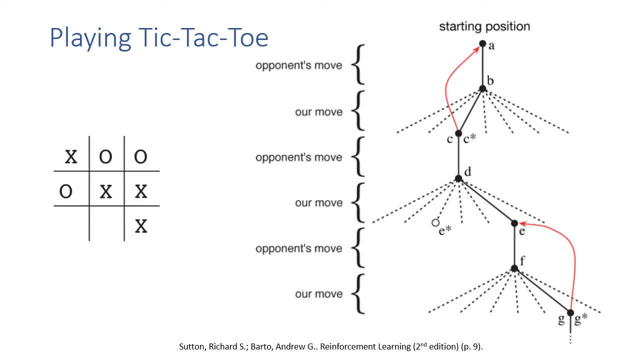 It's called the value function. We then play many games against the opponent. We move greedily, selecting the move that leads to the state with greatest value, That is, with the highest estimated probability of winning. Occasionally, however, we select randomly from among the other moves instead. 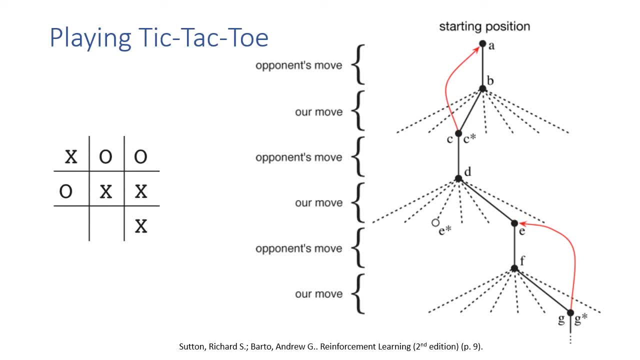 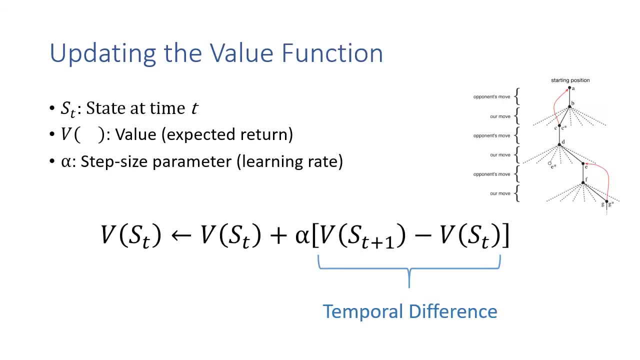 These are called exploratory moves because they cause us to experience states that we might otherwise never see. and let us learn other playing strategies. While playing tic-tac-toe, we keep updating the values of the states v of st. Higher value means that we have higher chance to win in the future. 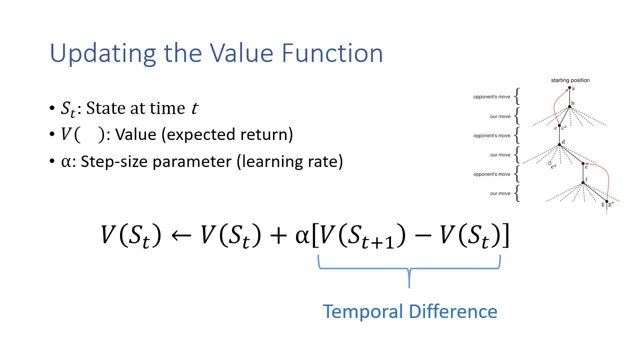 So our learning goal is to make the value more accurate, estimates the probability of winning. To learn the values, we would first play the game to the end and then back up. We need to play to the end to see if the result is winning or losing. 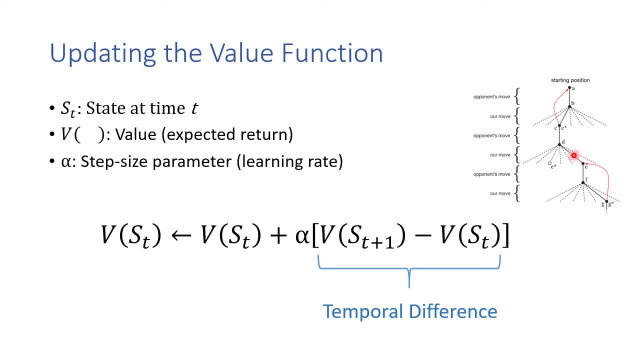 And then we back up, back up the value of the state after each greedy move to the state. before the move, The red arrows means the value update. Here is the formula of updating values. We will calculate the difference of later states: v of st t plus 1,. 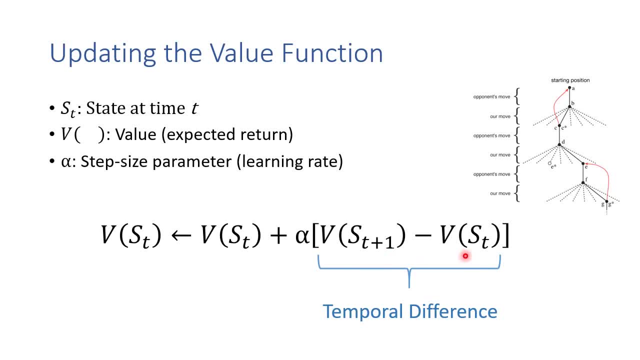 which means the future step of current state st. We will use the next step as t plus 1 minus the current value. This is called temporal difference And we will update the difference to our current state by a learning rate. So the basic idea of value function is to calculate the difference between the next step and the current step. 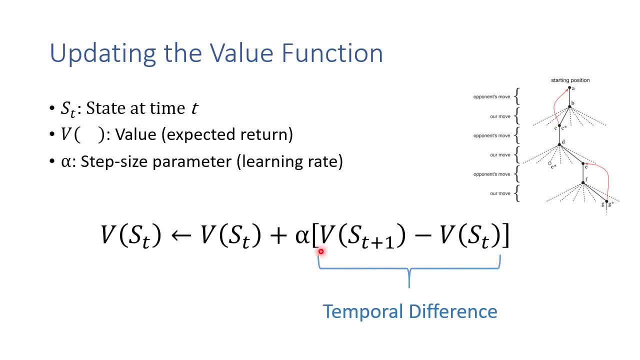 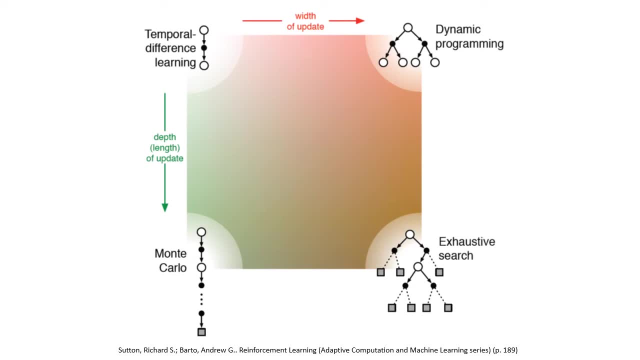 Then use the temporal difference to update our value function. All kinds of reinforcement learning algorithms can be viewed as a searching along width and depth of the MDP expanded tree structure. The record of each depth searching is called a trajectory. All reinforcement learning methods have three key ideas in common. 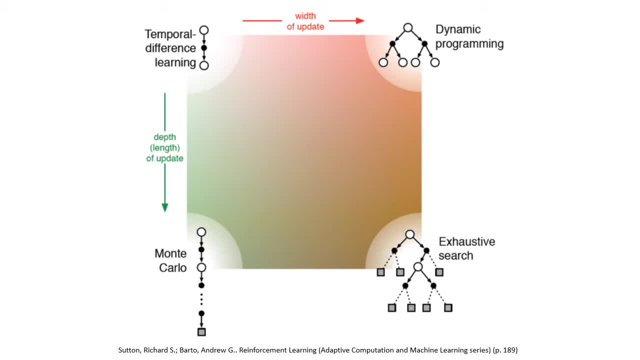 First, they all think to estimate value functions. Second, they all operate by backing up values along actual or possible state trajectories. And third, they all follow the general strategy of generalized policy iteration, Meaning that they maintain an approximate value function and an approximate policy. 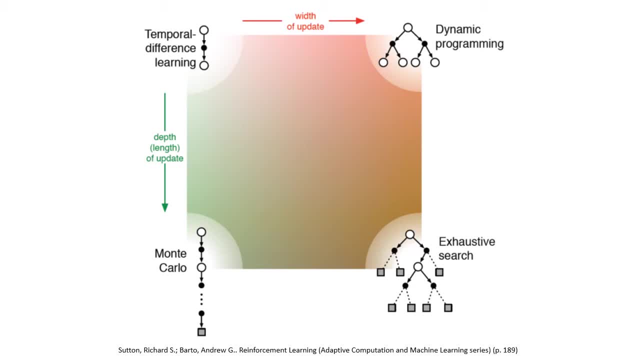 And continually try to improve each other on the basis of the other. These three ideas are central to the subjects covered in Sutton's book, which is the Bible of reinforcement learning. As shown in this figure, the most fundamental learning algorithm is temporal difference learning. 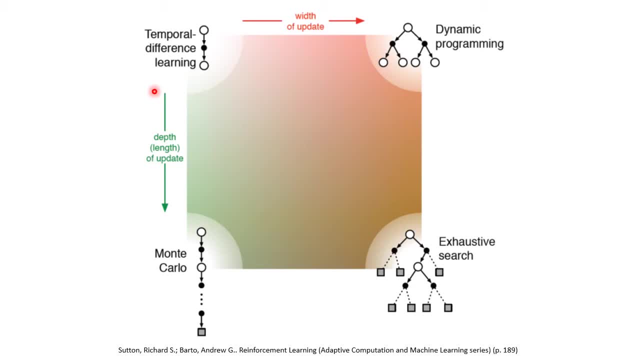 The formula of temporal difference learning has been shown in previous slides. If we decide to go to the depth first, to expand all the possibilities in the depth first, it's called the Monte Carlo method, For example, for learning chess. we would like to plan chess to the end of the game and back update the values of the previous value function. 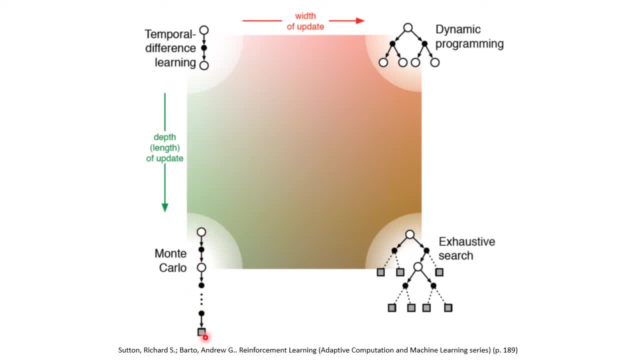 So for Monte Carlo method, we will plan to the terminal state and then back update all the value functions. Another dimension is width update, which means we will evaluate all possible actions at this state and then calculate, then updating the value function. This is called dynamic programming. 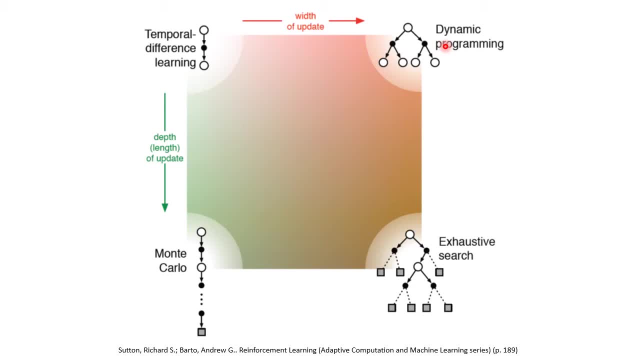 So updating the value function is very much like a search on a tree. If we decide to go depth first search, then it's called the Monte Carlo method. If we decide to do width first search, then it's called dynamic programming, which means we evaluate all the possible actions of this state, of current state. 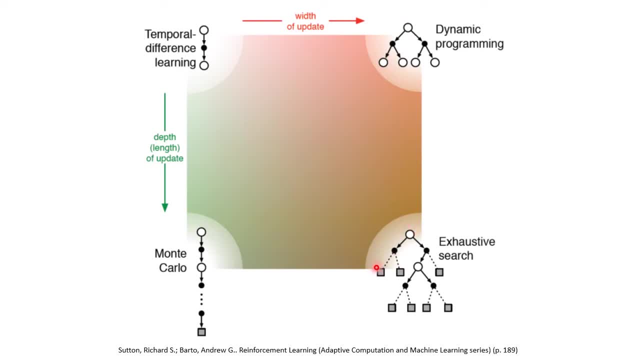 But if we have a lot of time and computing resources we can do exhaustive search to evaluate all the possible actions And all the next state, all the terminal state. This is called exhaustive search, But it's not practical in real applications. So usually we are choosing between Monte Carlo or dynamic programming. 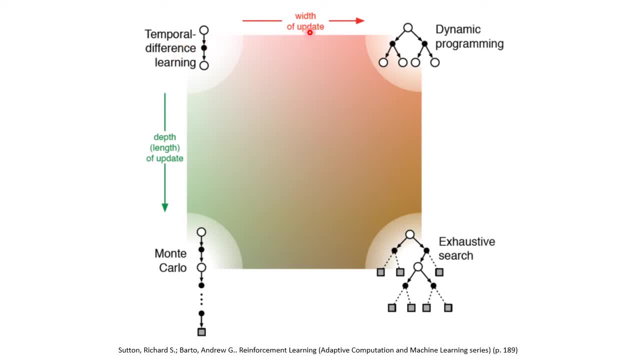 From different perspective. the horizontal dimension is sample updates, between sample updates, which is based on sample trajectories. So if we use temporal difference learning one step or multiple steps, we will have a lot of trajectories. It's called sample update. We will use the trajectory which is actually the experience results. 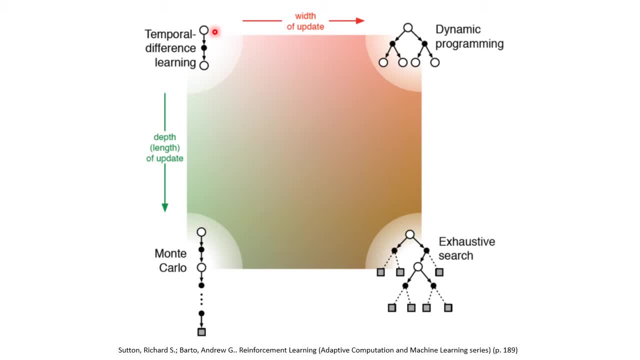 Playing result is called trajectory to update the value. Or we can use the expected value based on the distribution of the probability, So it's called expected update. But this requires an action probability distribution model. Why all the sample updates only need a sample model? 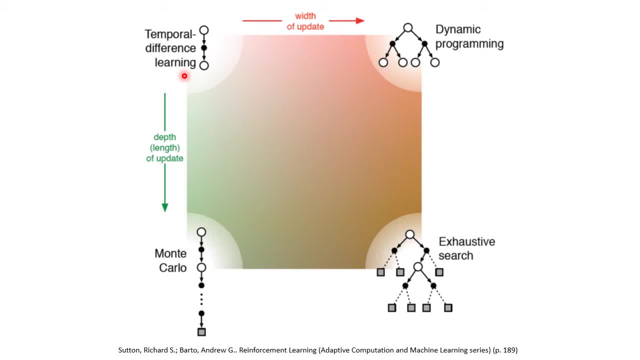 It can be done from actual experience with no model at all. The vertical dimension corresponding to the depth of update, that is the output strapping. So it's called bootstrapping because it will play the states by itself and back update the value function. 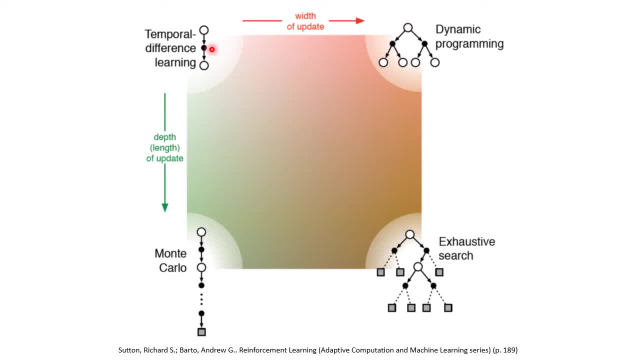 So at the three corners of the four are the primary learning methods, temporal difference learning, Monte Carlo and dynamic programming. The exhaustive search is just the extreme case that is running so deep that all the terminal states have been visited And we can calculate all the probabilities. 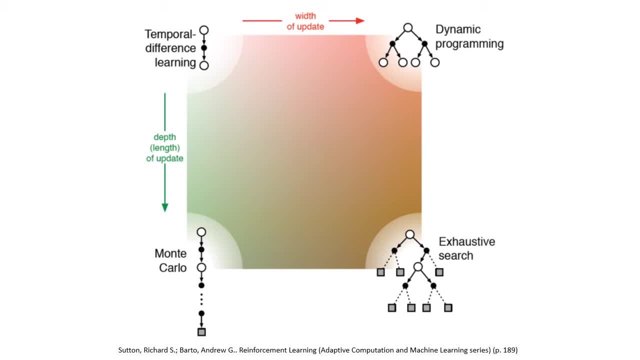 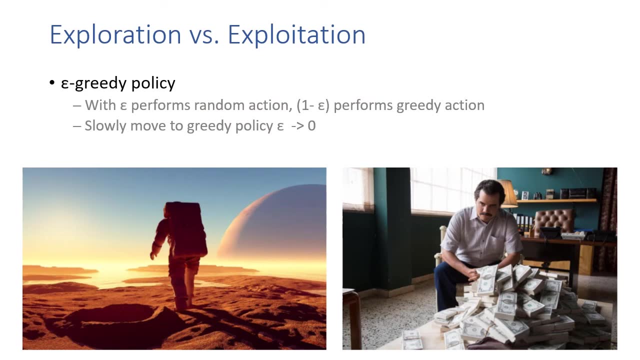 But it's just the extreme cases, not for real application. All reinforcement learning algorithms face the exploration and exploitation dilemma. Exploration means that the agent tries to search for new ways by taking random actions. Exploration means that the agent tries to search for new ways by taking random actions. 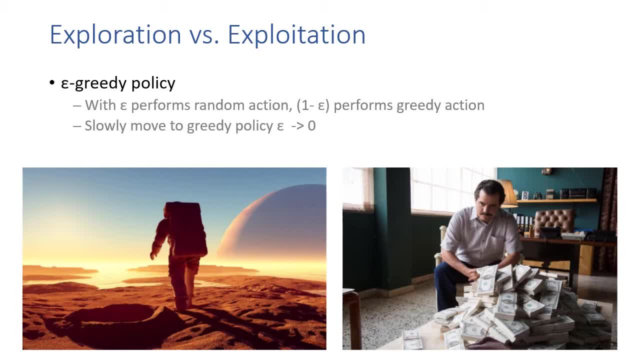 Exploration means that the agent tries to search for new ways by taking random actions. Exploration means that the agent follows current policy and selects actions greedily, that is, always select the current best action. Exploration tries to find better strategies, while exploitation focuses on improving current policy. 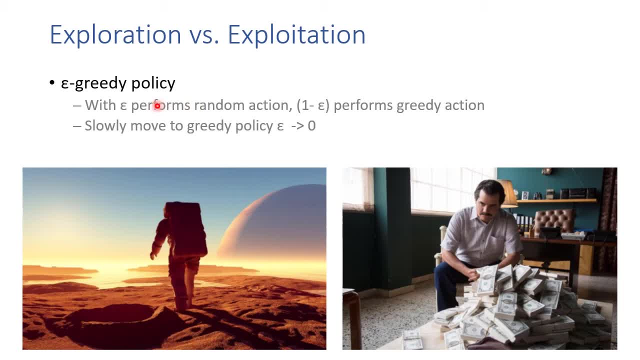 The most common method is epsilon greedy, which performs random actions, epsilon at a time time and perform the greedy actions one minus epsilon of the time. The figure to the left means the exploration, which means our algorithm like to explore new possible ways And the figure 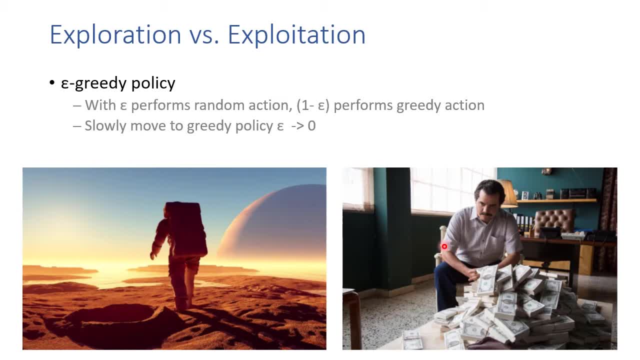 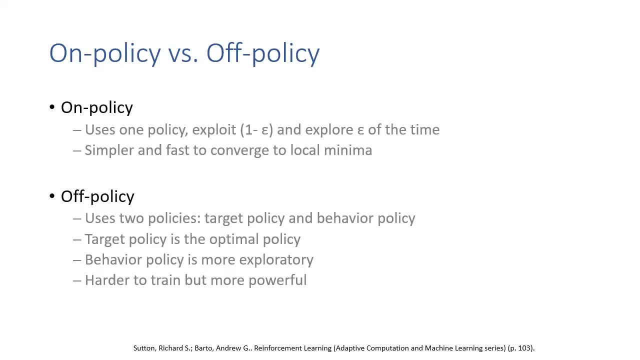 to the right means. exploitation, which means we select the best current approach. Selecting current-based action is called the greedy method. So there's a lot of money. this is a greedy method. Now we know that all the learning control methods face a dilemma. 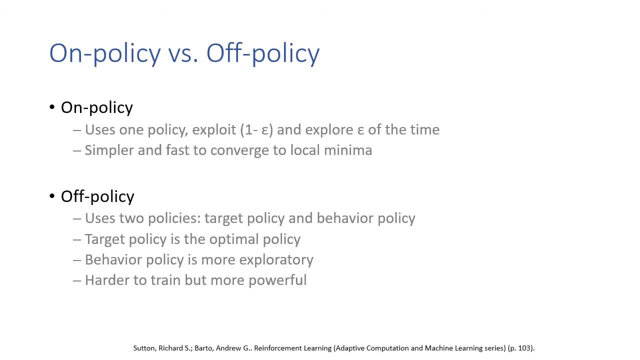 They think to learn action values conditionally on subsequent optimal behavior, but they need to behave non-optimally in order to explore all actions and find the other possible optimal actions. So how can algorithms learn about optimal policy while behavior behaving according to an exploratory policy? So there are two kinds of learning policy. The first is unpolicy. 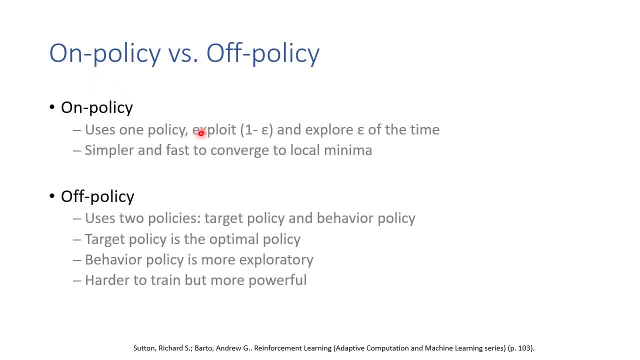 Unpolicy means that we use a greedy algorithm, epsilon greedy algorithms, which means we have epsilon readiness to explore. We have to explore random actions, epsilon of the time. But it's actually a compromise. It learns action values not for optimal policy but for near optimal policy, But it's simpler and 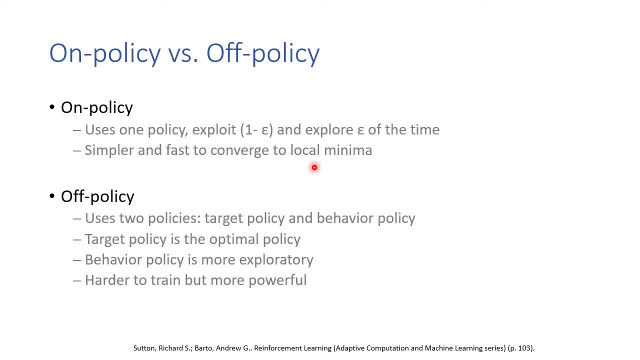 fast to converge, However, to local minima. it's more difficult to find global minima, So it tends to converge to local minima. On the other hand, there's another approach, called of target policy. Our policy is actually used to policies, target policy and behavior policy. 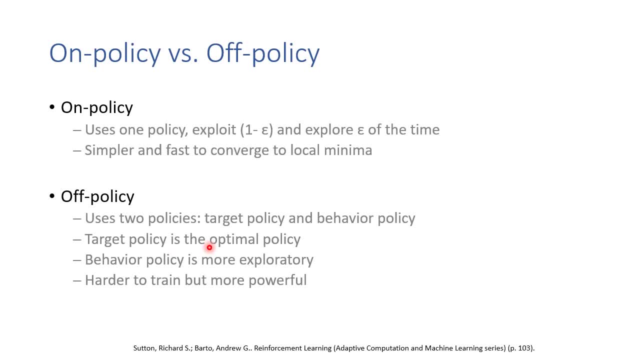 So target policy now is our current optimal policy, current best policy, And the behavior policy is more exploratory. So we allow the behavior policy to try more different random actions and update to the target policy after a period of time. This is called of policy, because the learning is from data, of of the target policy. 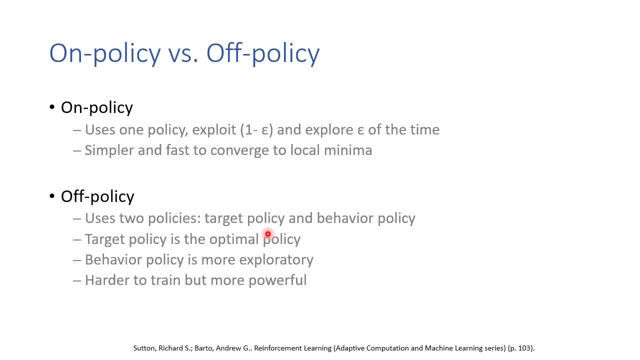 So the overall learning is used to policy. So it's harder to train because we have two policies now, but it's more powerful in the long run. In the beginning the unpolicy may converge faster and have better performance. In the long run the unpolicy will get better performance. 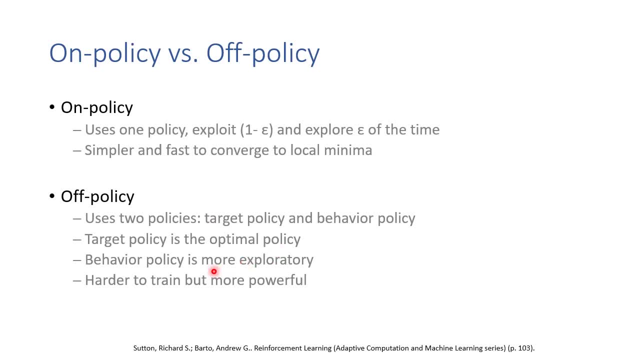 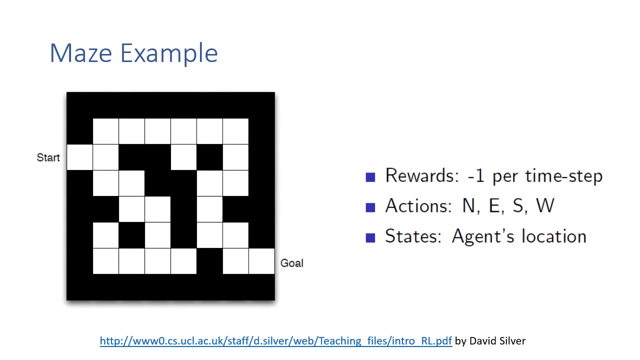 because it can keep the optimal policy while let behavior policy to explore more options. Let's look at a math learning example. This example is from the first class of David Silver's reinforcement learning. The objective of the agent is to find the shortest path between start and the goal. Here's the possible shortest path. 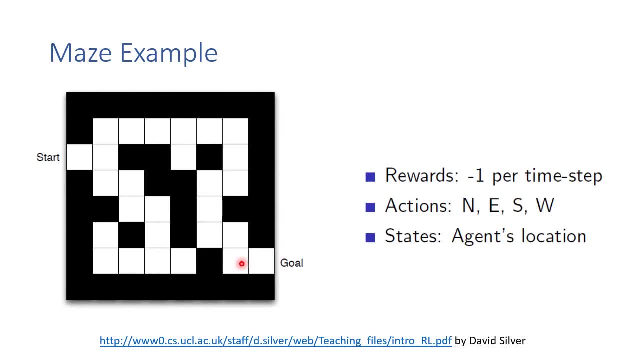 To let the agent learn the shortest path, we will give the agent minus one reward- negative reward per time step. So it encourages the agent to arrive at the goal at the shortest time, which means it will have less minus reward. There are four actions: moving north, east, south and west. The states are the agent's location. 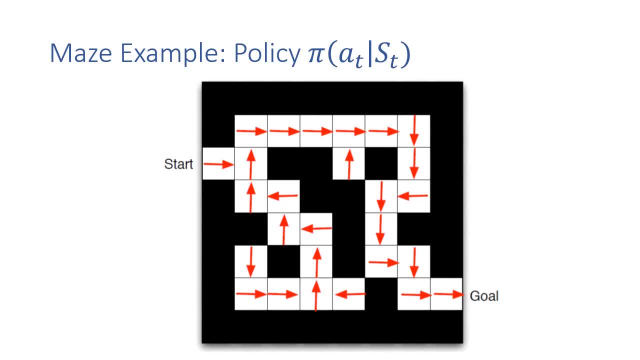 Here is how the policy function looks like: A visualization of policy pi of at under the condition of state t. In this example, the red arrows are the actions. the red arrows are the actions of the agent. Choose to do under different state. This is a deterministic policy. 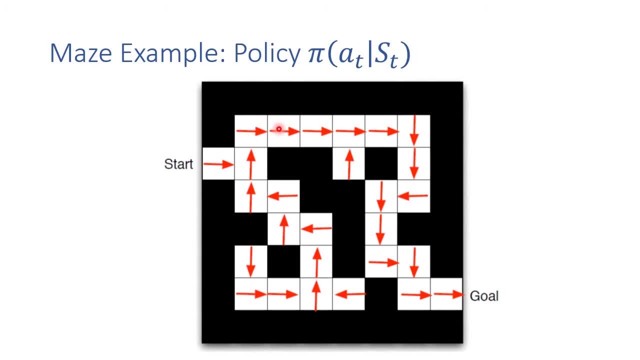 which means we always select one specific action at a specific state. So if we learn the model, we train the model successfully. the policy model will show us which action has highest probability to achieve a long-term highest value. So follow the direction of the policy model. we can find the shortest path. In this case, this is a policy function. 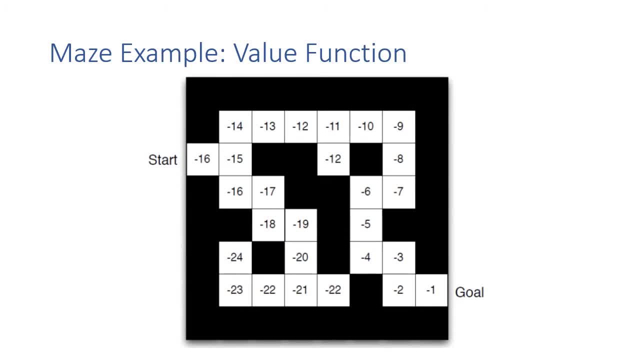 On the other hand, we can learn the value function of each location and use the value function to choose our action. Let's look at the value function of the map. We can start from the location nearest to goal. We have minus one reward because it will take only one step to reach the goal. 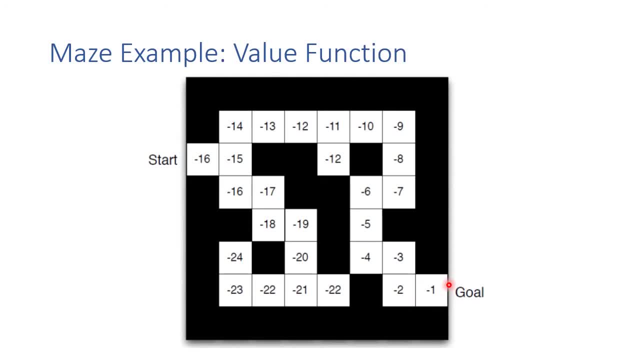 So only one step. we can reach the goal. The value is minus one reword. By moving toward the location of a higher value, we can find the shortest path. In this case, the second location is minus two because it takes our takes us to two. 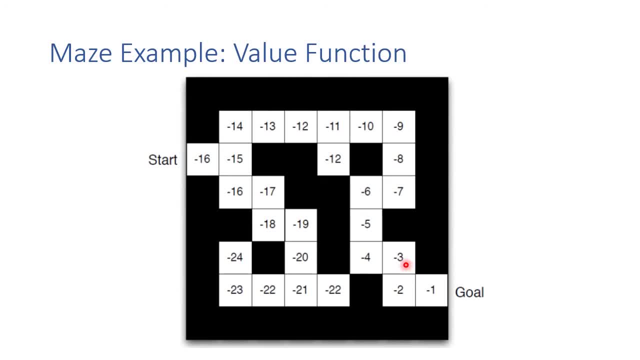 step to reach the goal. the goal right, minus 3,, minus 4.. So the star has very high minus value: minus 16.. So now we suppose we our edges start to work to the goal, then we will choose. 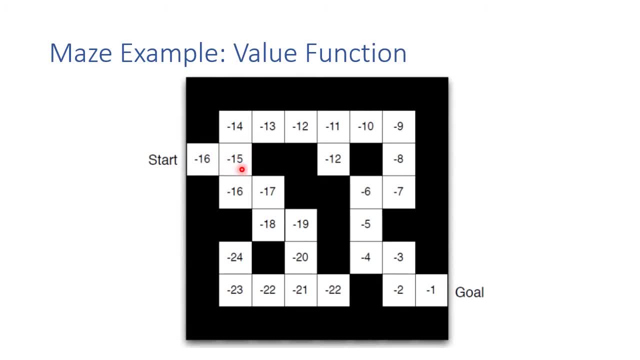 the position that has highest value, which is the minus 15, and then, in this position, we will choose the next position with highest reward, which is minus 14,. then follow this value function, follow the greedy policy. we will always choose the one with highest reward. We can also find the shortest path. 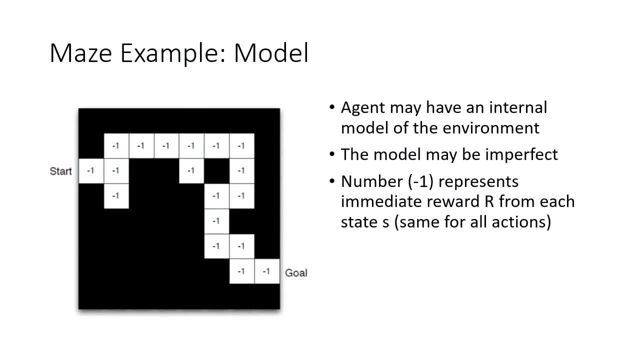 The third approach is to build an internal model of the environment for the values, which is very much like drawing a map by exploring the environment. In this case, the agent built an internal map of the environment and then the agent can find a way to the goal. 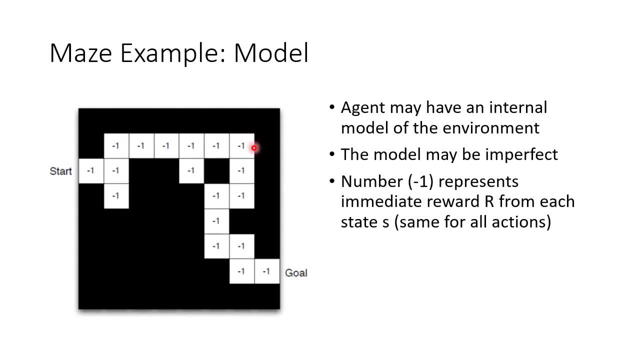 For example, after hundreds of tries the agent may find a path. This is called a trajectory, a trajectory of reaching a goal and give each step a minus one reward. So once we have an internal model, we can use the model to explain, to plan the shortest path. 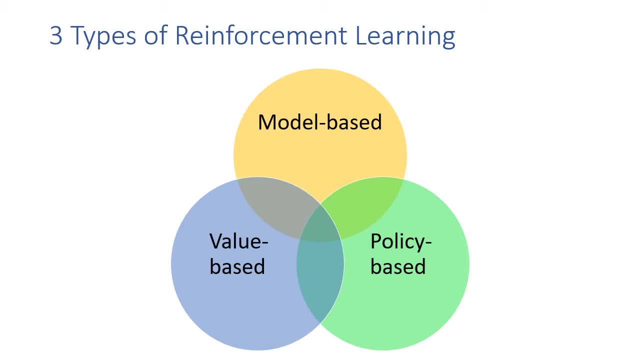 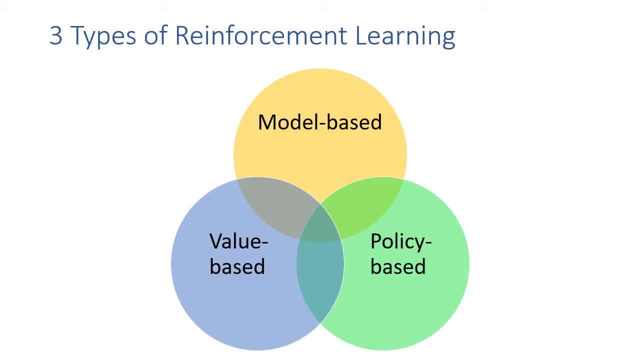 The model-based methods, the value-based method and the learning algorithm. Most reinforcement learning algorithms are model-free and belong to value-based or policy-based, such as DQM belong to value-based and the policy gradient is a policy-based method. Some algorithms are mixed of two types, such as actor-critic. If we have a good model of the 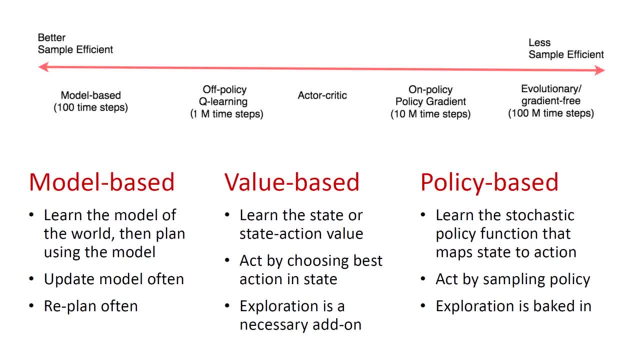 environment. then we can use the model to plan the actions and the learning will be very efficient. We may just need to play in an environment 100 times- It's called time steps, 100 times steps- and achieve the good result. However, it's difficult to learn the model of a complex 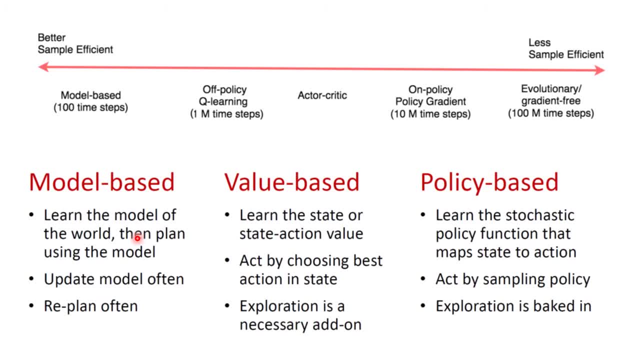 environment in practice. So usually we prefer other tools. The model-based methods, the value-based method learn a possible reward which is called the value of each state or even the state action value. It can learn the state value or the state action pair. 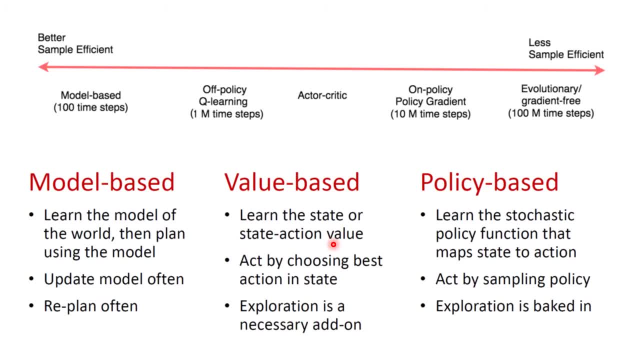 value And then we can act by choosing the best actions. which has highest value in next state? We need to add exploration in the value-based method For our policy: Q-learning. we may require around 1 million time steps to achieve good results. So value-based- we need more training. 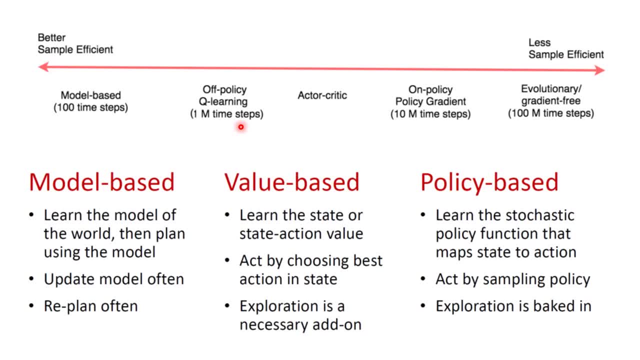 steps and the model-based method. The third method, policy-based method, is directly optimize the policy function. The third method, policy-based method, is directly optimize the policy function. The policy function will generate the probability of selecting actions, so we just act by sampling the probability output of our policy function. 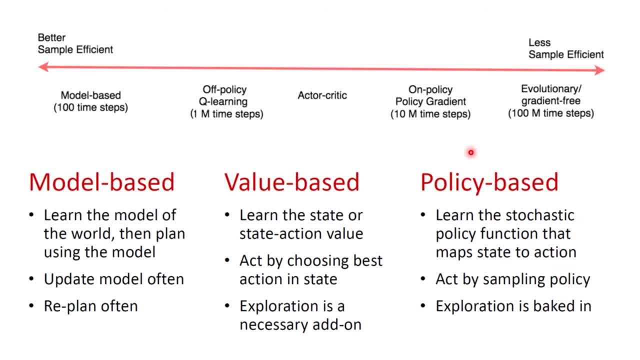 The exploration is backed in now. However, the policy-based method requires much more training steps. Like the un-policy policy gradient method, this requires around 10- 10 million timestamps. for other algorithms it requires 100 million times step two to achieve acceptable results. 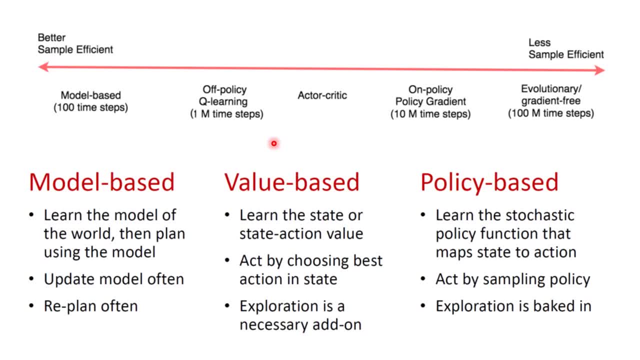 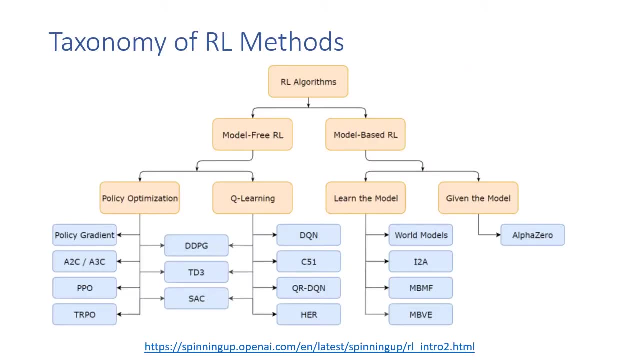 and the. the popular method now is the mix of value-based and policy-based, called actor-critique, and this is a balance between the value-based and the policy-based method. this is the reinforcement learning taxonomy from OpenAI. this tree diagram includes most. 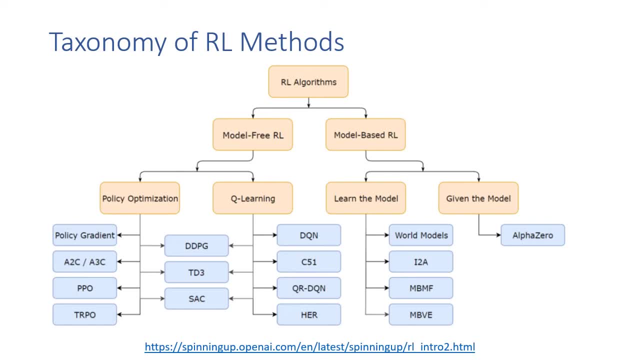 state-of-the-art reinforcement learning algorithms. OpenAI classify model first classify algorithms into model-free and model-based. the policy optimization and the Q-learning belong to model-free reinforcement learning. the most famous Q-learning-based algorithm is the deep Q-learning DQN. other popular algorithms of policy optimization. 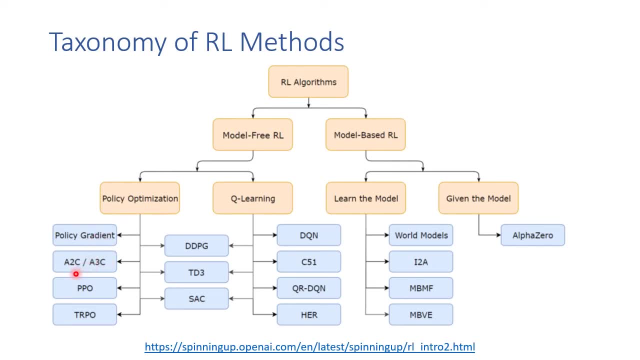 include the policy gradient and the actor-critique method, asynchronous actor-critical method, A3C is the asynchronous actor-critique agent and A2C is synchronous actor-critique agent. those are very popular methods for model-based reinforcement learning. there are word models or other algorithms. 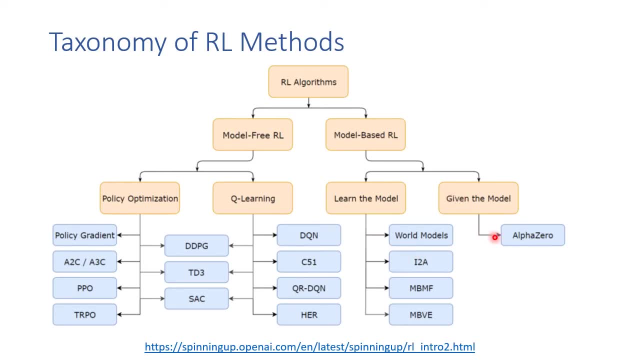 one special case is alpha zero or alpha go, which are given the model because we know the rules of the of the game go right and the chess games are fully observable. so chess games are actually. we have the model of the chess games and they are simplified. learning problem: 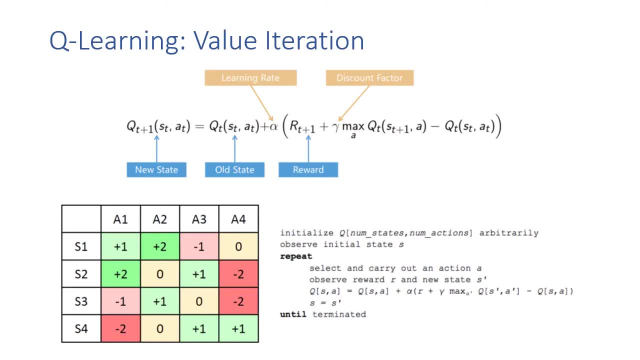 let's introduce the most popular value-based method, Q-learning. Q-learning learns the values that can estimate the expected future reward for different actions under various states. we can formulate it as a Q function of state and action. Q refers to the quality. we can update the. 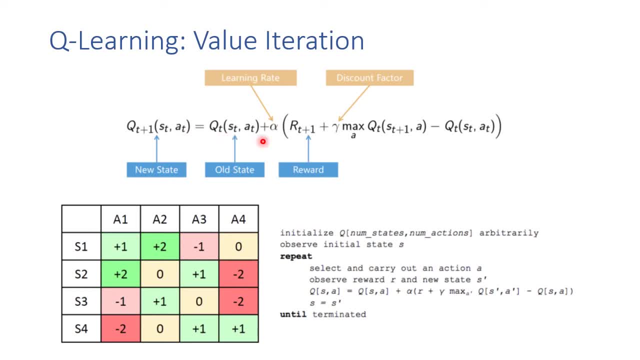 Q function using Bellman equation. it's very much like the temporal difference learning. however, note that we use the maxima value of our next step, Q value, as our target, so this is an off-policy learning method. if the number of states and the number of actions are few, we can build an action state table. 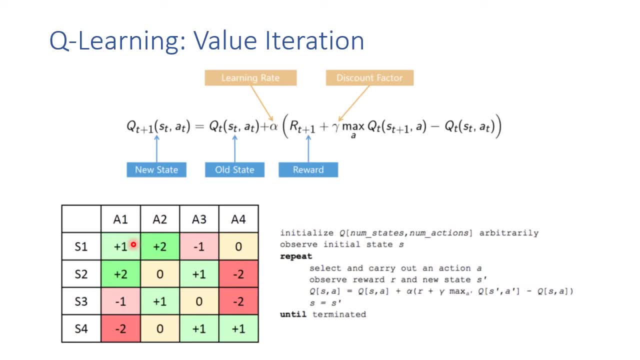 here is the action state table, which is also called Q-table, to calculate the corresponding rewards of each action and the state pair. as shown in the lower left corner, however, the number of states are very large in real world. it is inefficient and nearly impossible to build a complete action state table. 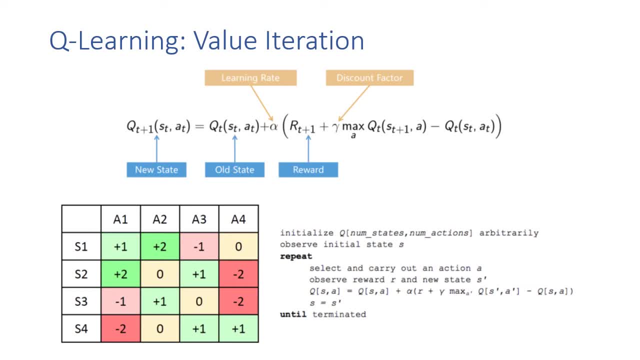 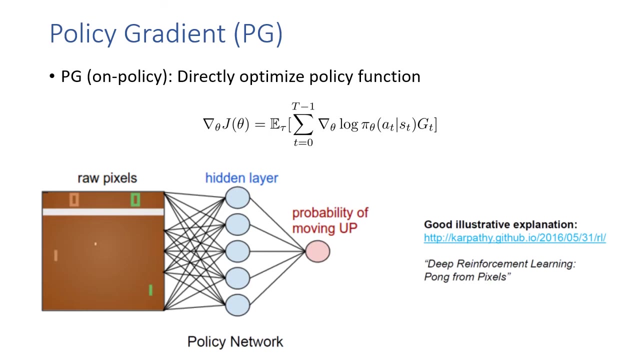 so deep mind solve this problem by using neural network to the Q table. Their method is called deep Q learning- DQN. About policy-based method, the most popular algorithm is policy gradient. Policy gradient is an intuitive method that directly optimize the policy function. This is an unpolicy function because we only have one. 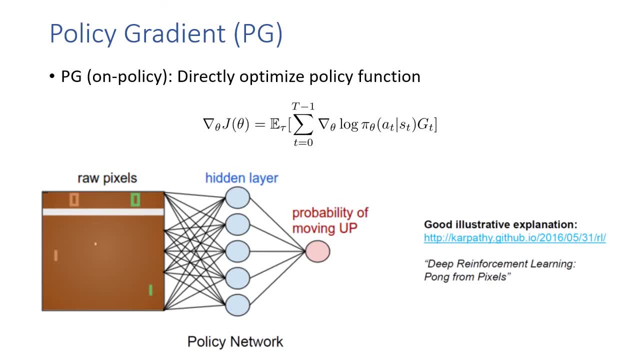 policy function. Compared with the off-policy methods such as DQN policy gradient is easier to train and converge but also tends to stuck at local minima. Andrii Kapravi has made an very interesting introduction experience of training agent to play game pump using policy. 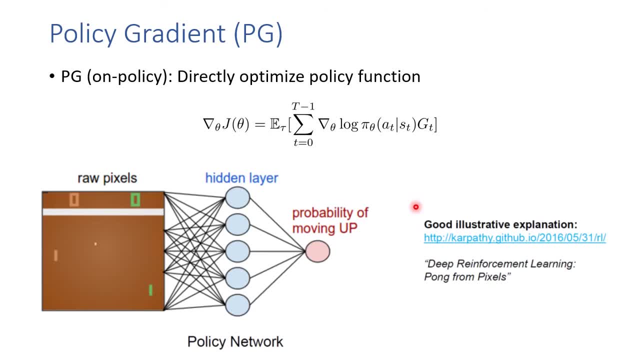 gradient. For more details you can refer to his github. Here is the formula of policy gradient. We usually calculate the log version of the policy function, which is usually a softmax, because softmax can give the probability of each action under different states. So we get the log version of our policy function and then calculate the gradient. The final log function we have is the gradient. So we get the log version of our policy function and then calculate the gradient. The final laws function is an intuitive formula which uses DQN. About policy gradient is an intuitive method which usually serves to train and converge but also tends to stuck at local minima. Andrii Kapravi has made an interesting introduction experience of training agent to play game pump using policy gradient. For more details you can refer to his github. 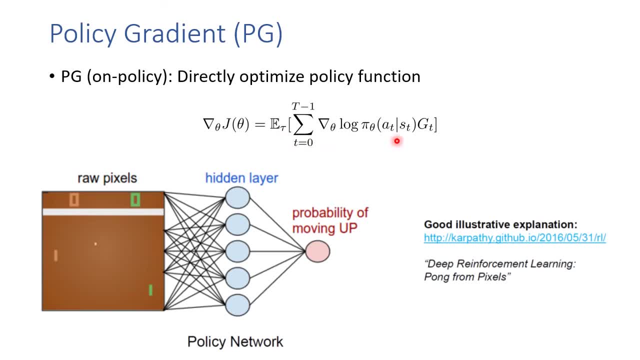 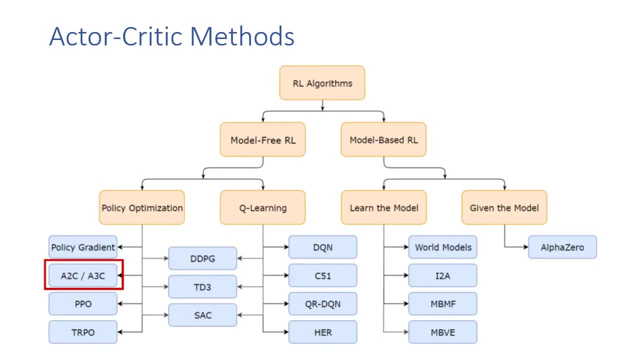 is the expected value of the policy gradient. so this is the policy gradient formula. another important branch of reinforcement learning is the actor-creative method. the two most famous actor-creative methods are a2c and a3c. let's take a look of those algorithms at next page. 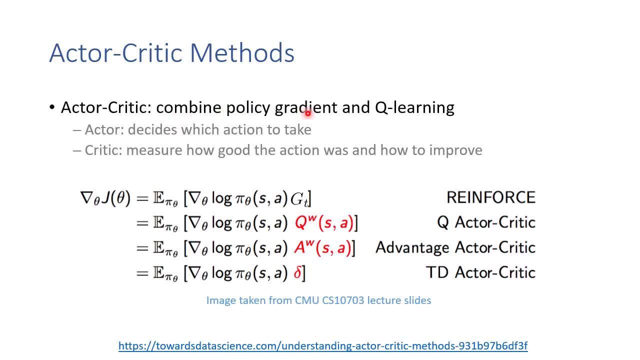 the actor-creative method combines the policy gradient and the q-learning. in other words, it combines the value-based method with the policy-based method. so there are two parts: one is by actor, which decides the actions to take under different states, and another one 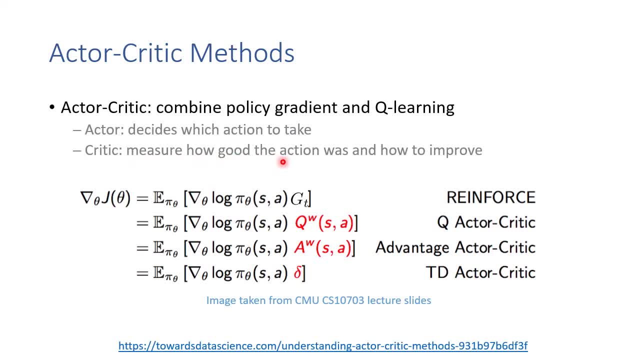 is critic. critic measures how good the action was and how to improve. this depends on the types of the value function. the actor-critic method can be classified as q-actor-critic, advantage-actor-critic or temporal difference of td-actor-critic. 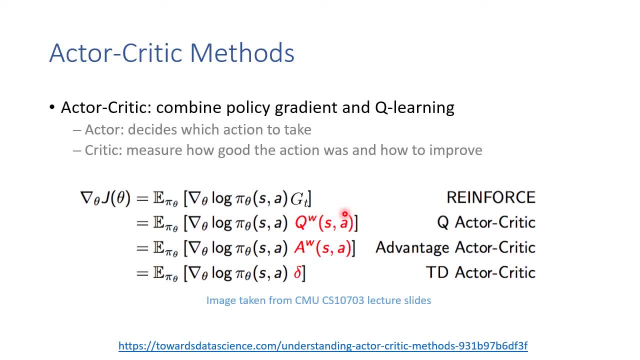 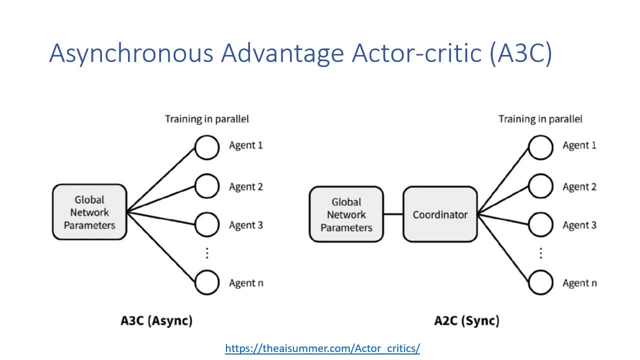 based on the value function we use. deepMind proposed the asynchronous advantage-actor-critic method, also called a3c. deepMind proposed the asynchronous advantage-actor-critic method, also called a3c. there is a global network, parameters and there are a lot of agents training in parallel. 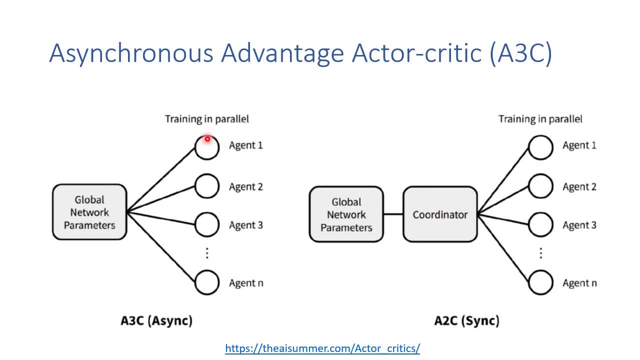 multiple agents learn parallelly in their own copy of environment and then update the global network periodically. the updates are not happening simultaneously, so that's why it's called asynchronous. after each update, the agent resets their parameters to those of the global network and continue their independent. 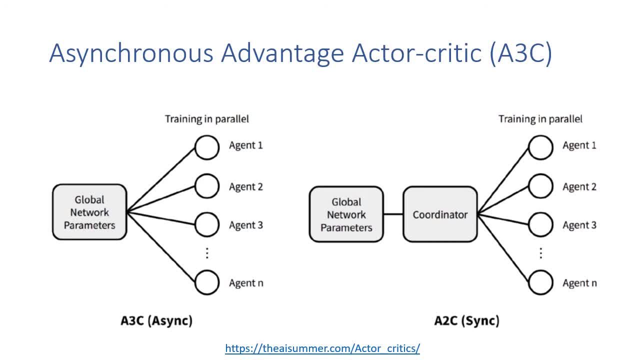 exploration and training for n steps until they update themselves again. we see this information flow not only from agent to the global networks but also between agents, because all the agents experience will part to partly be added to the global network parameters. so the a3c can: efficient learning on the multi-core computer for a3c. 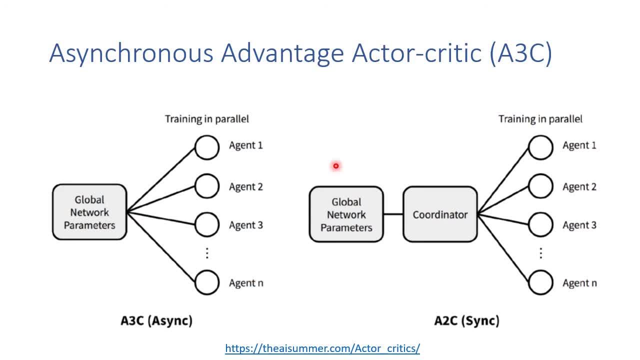 we usually use cpu to train the agents, not the gpu. on the other hand, the openai suggests that synchronous update may be more efficient, but we need to add an coordinator. this algorithm is named a2c because it's now synchronized version. it's synchronized. 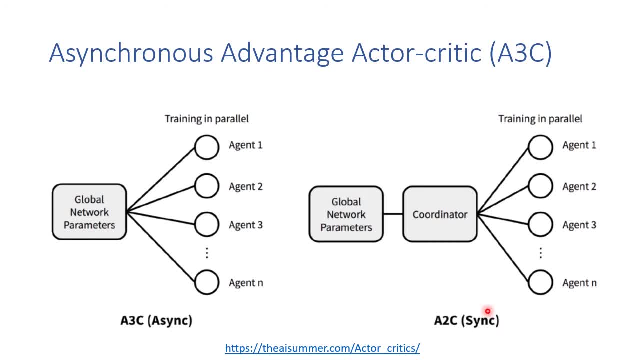 advantage-actor-critic- a2c. a2c outperforms a3c on many different projects. A2c is the only algorithm that we use to deploy a3c on a3c. a2c outperforms a3c on many different projects. 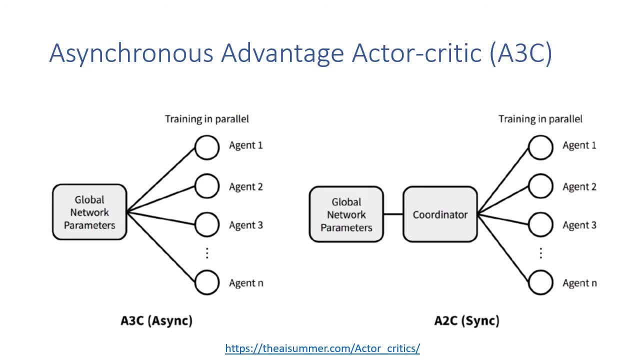 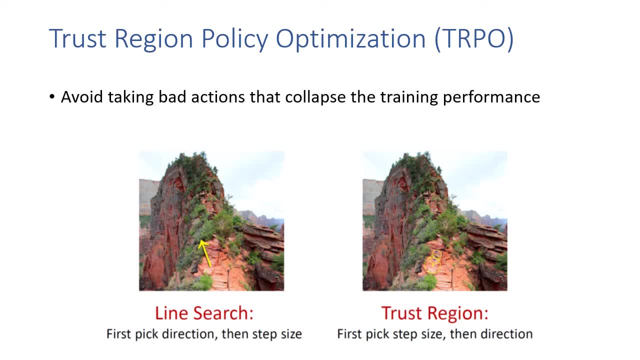 many reinforcement learning benchmarks. Training reinforcement learning model is very difficult, like other deep learning models. Here is a trick called the trust region policy optimization which can help to stabilize reinforcement learning training. The idea, or the basic idea, is to avoid taking bad actions. that 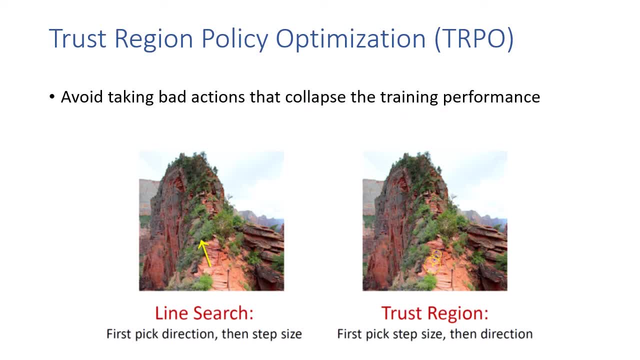 collapse. the training performance TRPO updates policy by picking up step size that satisfy a spatial constraint on how close the new and old policies are. The space is called trust region. The constraint is expressed in terms of pair-L divergence, a measure of distance between probability distributions. 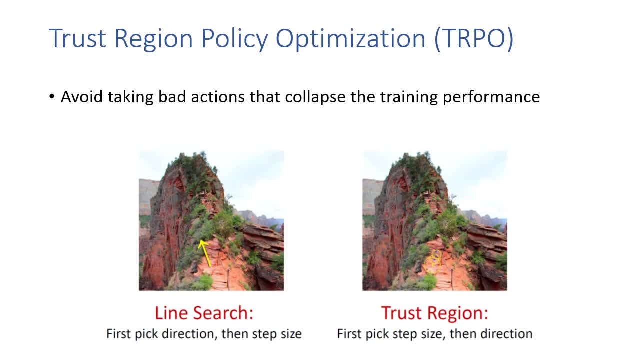 This is different from normal policy. TRPO has a policy gradient which picks a direction first, then step size. In practice, a single bad step can collapse the policy performance. This makes it dangerous to use large step size with traditional policy gradients- TRPO. 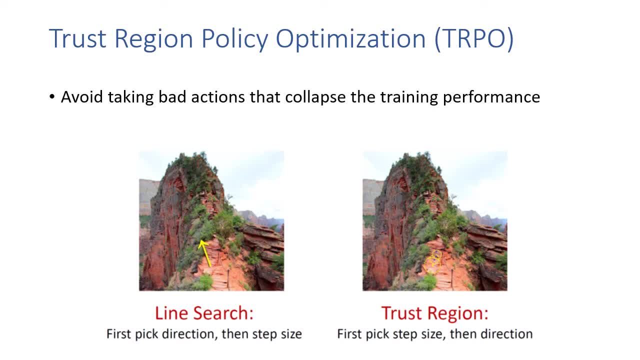 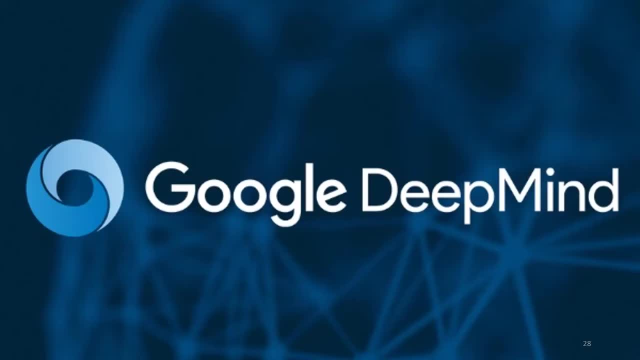 nicely avoids this kind of collapse and attempts to improve the performance quickly. In previous slides we have learned the basics of reinforcement learning. Now let's talk about the reasons advanced in deep reinforcement learning. Deep reinforcement learning are largely made by the DeepMind company. DeepMind was founded by David Hasselbeck, Shane Legge and 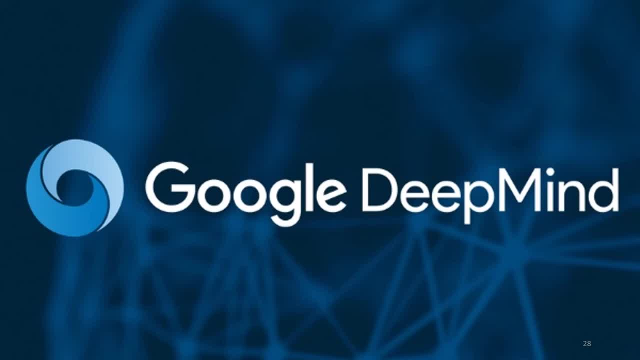 Mustafa Suleiman in 2010.. The goal of the founders is to create a general-purpose AI that can be useful for deep learning. The goal of the founders is to create a general-purpose AI that can be useful for deep learning. The goal of the founders is to create a general-purpose AI that can be useful for 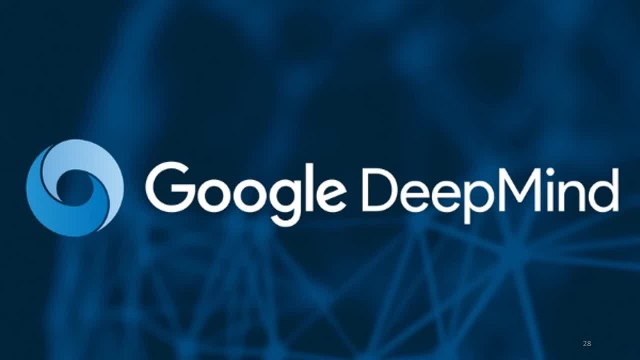 and effective for learning almost anything. Because the founders has a background in the game industry, they started training AI agents how to play old Atari games that were popular in 1970s and 80s. On January 26 of in 2014, Google. 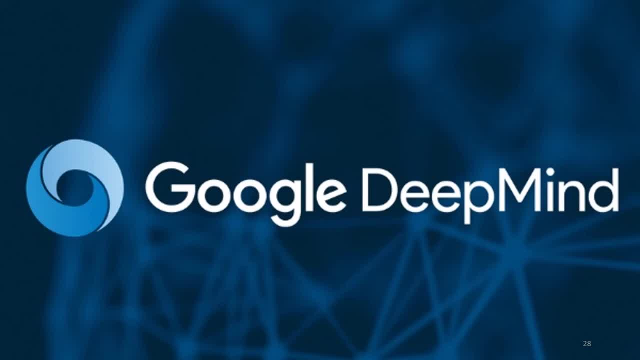 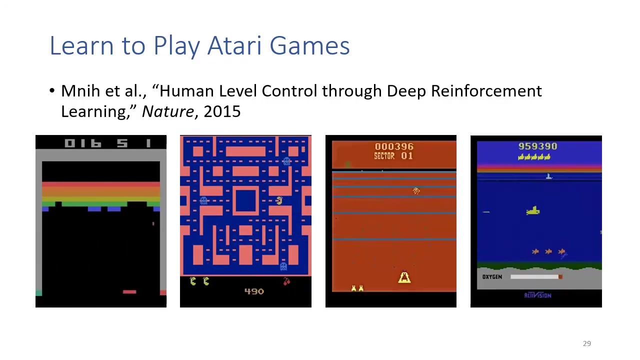 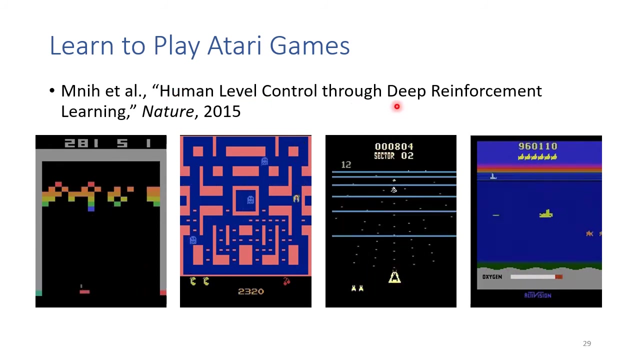 announced the company has acquired DeepMind, for The company made headlines worldwide in 2016 after its Avago program beat a human world champion, gold player, Lee Soo Dong. DeepMind published their first breakthrough algorithm: Deep Q-Learning. The title of the paper is Human-Level Control Through Deep Reinforcement: Learning in 2015.. 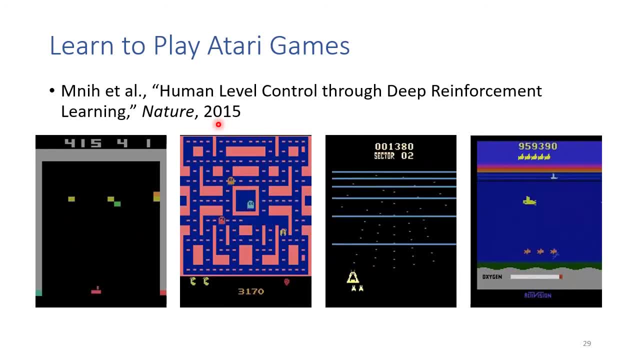 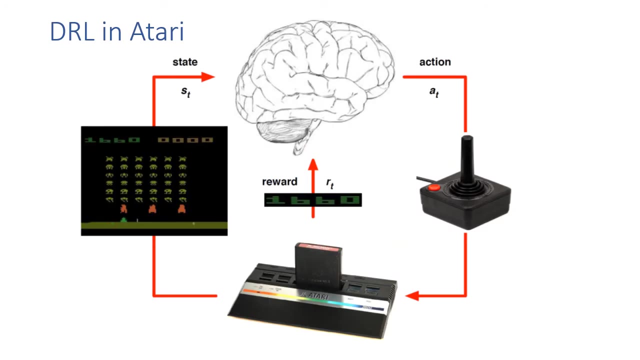 Here are some examples of AI playing Atari games in OpenAI Gym. OpenAI Gym is an open-source reinforcement learning simulation environment released by OpenAI. We will use OpenAI Gym to try some algorithms later When training and training AI playing Atari games via reinforcement learning. 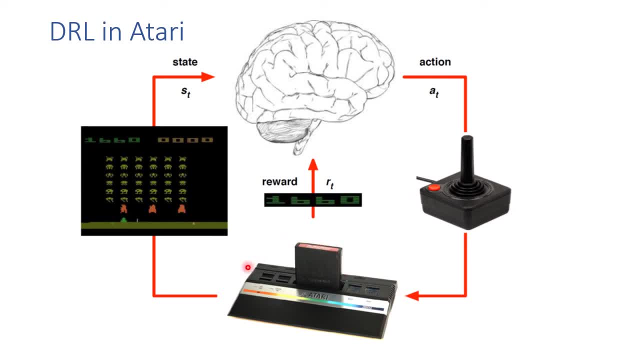 The environment is Atari Game Console. Here is the picture of the Game Console, which was made in 1970s, And the reward is the score of the game And the state is the screenshots. The actions are the directions of buttons. you can see the buttons of the joysticks. 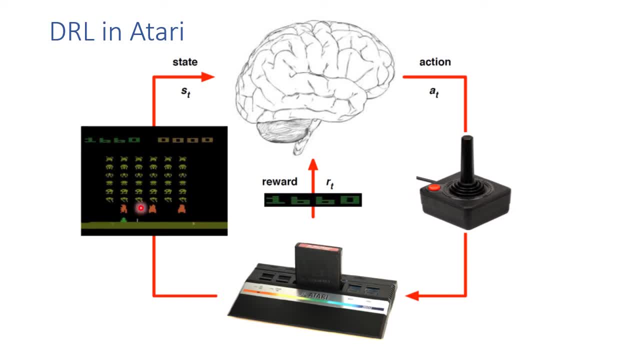 The very ambitious. They want to create a general intelligent intelligence. So they didn't preprocess the game screenshots, They didn't try to label the objects or enemies, They just send the state, the whole screen, into the, into the model. So they just use the use the raw pixels of the screen. 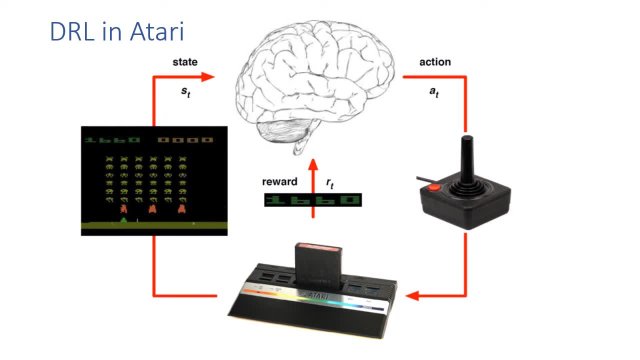 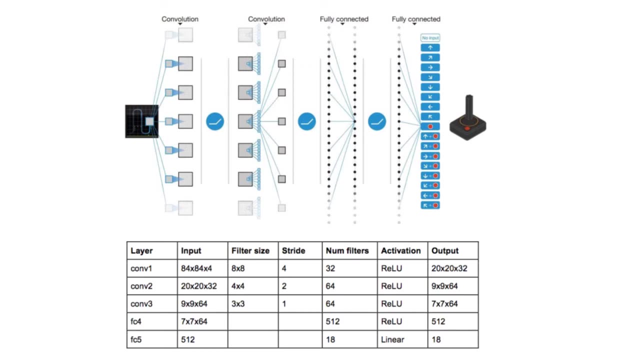 And they hope for future, use screenshot as their input, as their state. so this makes the possible states very huge. the number of possible states is very large. the breakthrough of DeepMind's deep Q-learning is to use neural network to approximate the Q-table. 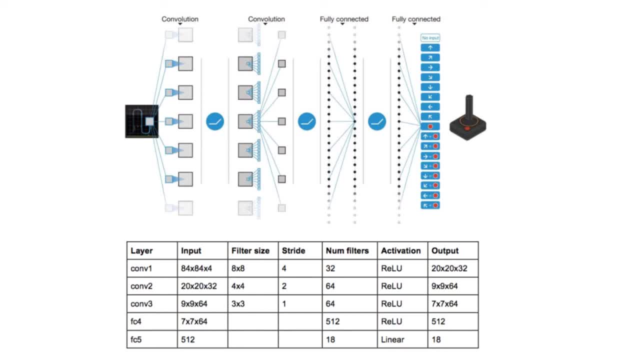 DeepMind adopted a small neural network that has only three convolution layers and two connected layers, two fully connected layers. surprisingly, a simple network can successfully learn many different Atari games and achieve human-level performance. here is the table extracted from their original paper, which shows the parameters of each. 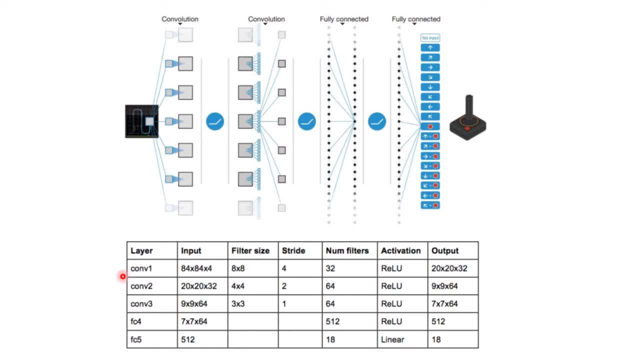 convolution layer and the fully connected layers. so for convolution 1, the input size is 84 by 84 by 80.. the input size is 84 by 80.. the input size is 84 by 80.. the input size is 84 by 80.. 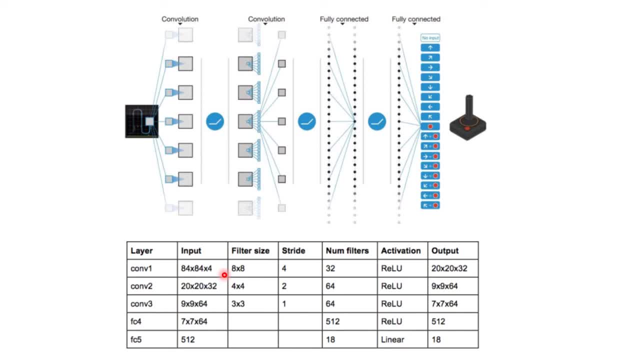 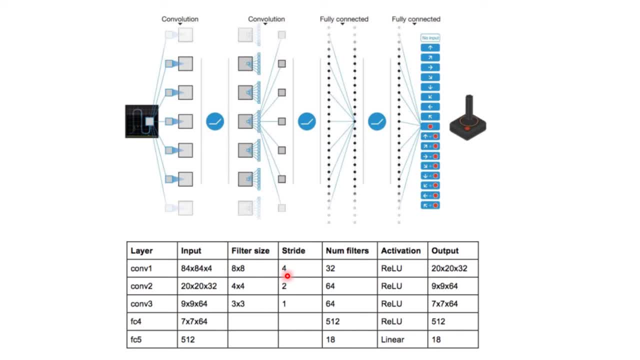 reduce the size. also, they first use a large stride- okay, as common. the number of filters increase with the depth of the layers. the final output dimension is 8, which are directions plus the fire button. so there are 18 output selection. 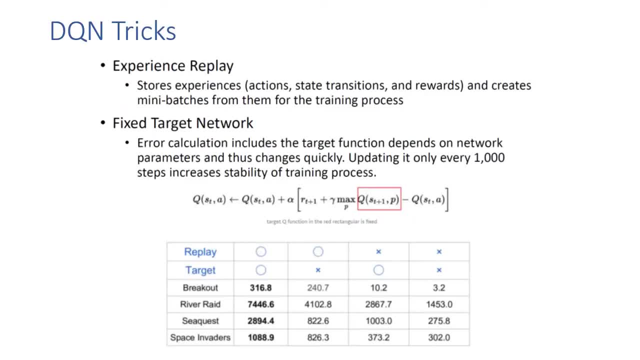 both reinforcement learning and the neural networks are hard to train. DeepMind introduced two tricks that make training DQN stable. the first trick is experience replay, which stores the previous action between states and rewards, which are called trajectories, and provides the name again for 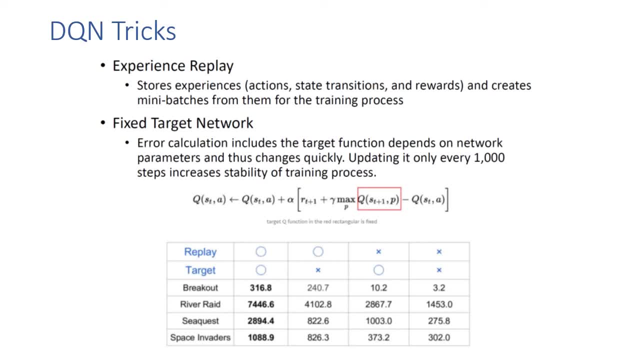 later training. this trick allows DQN to review important actions and decouple the high correlation of continuous actions. the second trick is to use of policy strategy so they have a fixed target network which can separate learning into behavior policy and target policy. they update the target network. 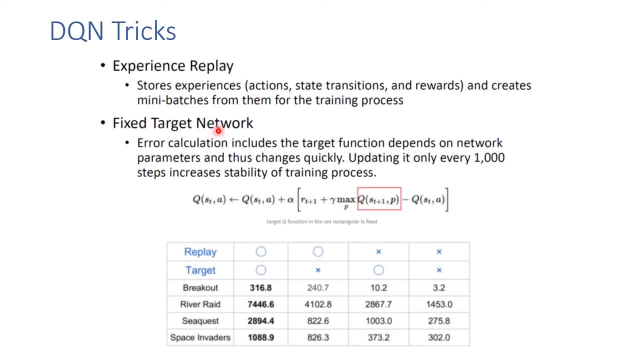 every 1000 steps. in other words, if we only have one network, calculating the network will depends on. depends on the network parameter can change quickly and is unstable. updating it every 1000 steps increase the stability of training process. actually, as we know, Q-learning is a of policy network. so 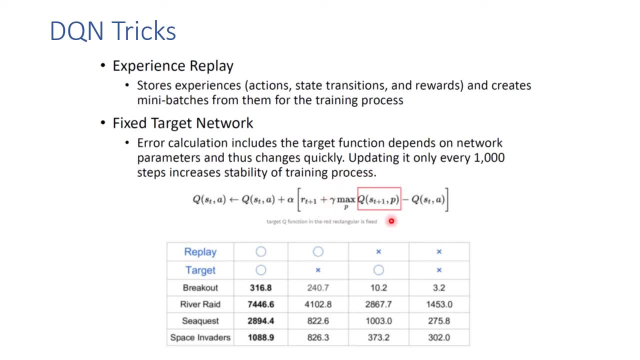 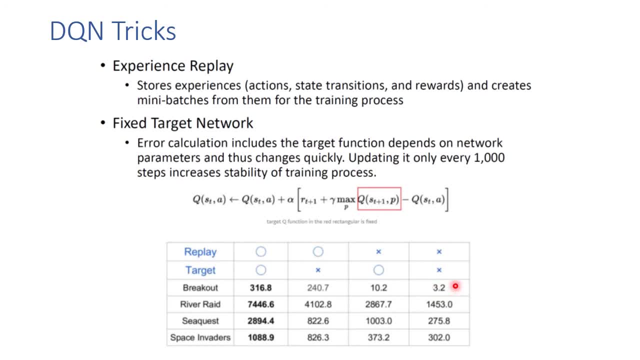 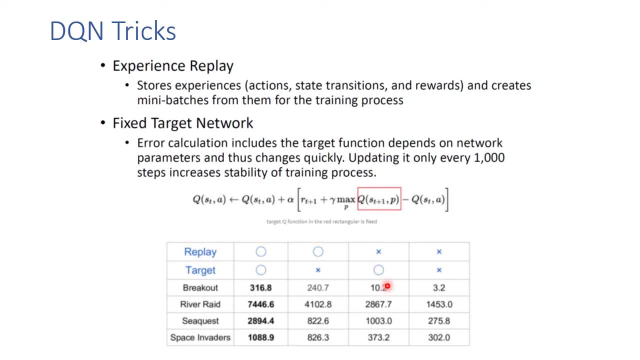 but we improve the performance of Q-learning. therefore, it will improve our performance, improve the performance, improve our practicality. we can also control our brain, but it doesn't allow you to control the brain, so we have a cycle sequence of mentorship很好魔学和他龙. 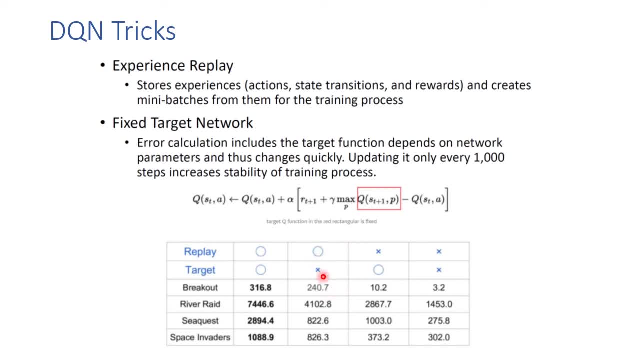 Gosh, I am just пережived that the Chinese teacher looks at me miserably because I should like to introduce him to this lesson. so please remember, this is a traditional method and we are learning it step by step. it's easy and it's easy. 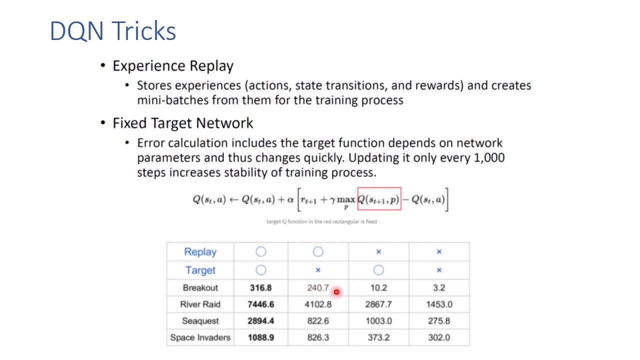 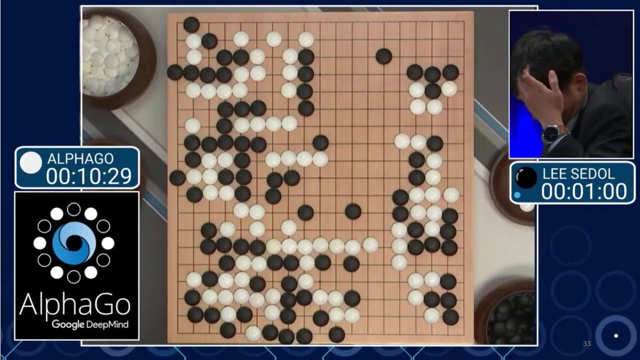 40 or so. it works with experience replay, so it's very tricky. if the author didn't find those two tricks, it can. only the deep learning or the e-learning works model cannot be trained successfully on Atari games. the most famous success story of DeepMind is about Go. 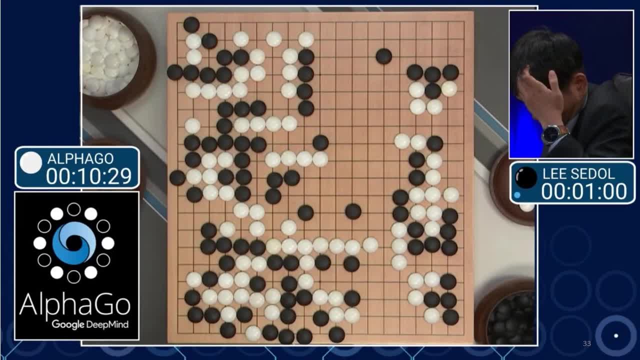 in 2016,, AlphaGo won the five-game goal match against the 18-time world champion, Lee Soo-dong and lost only one game, which is the last game won by human after AlphaGo. after this match, AlphaGo has sweep the human opponents. 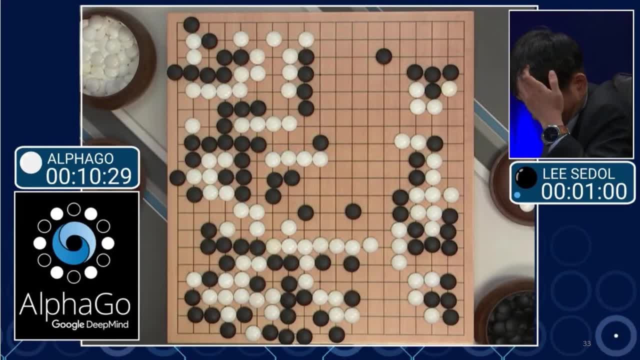 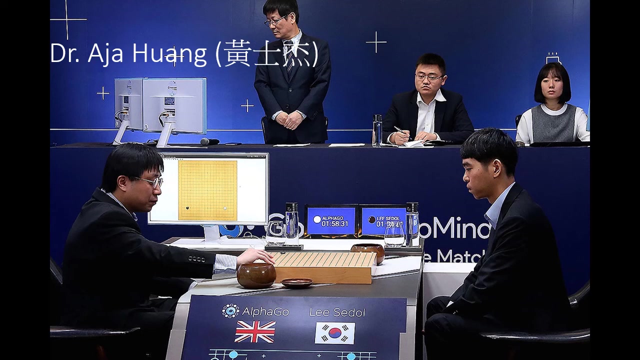 no professional goal player can win AlphaGo right now. Go was considered the holy grail of human intelligence because previous algorithms can only beat mature players. this is indeed a great achievement in human history. actually, there's one Taiwanese that work for the AlphaGo team. his name is Aja Huang. 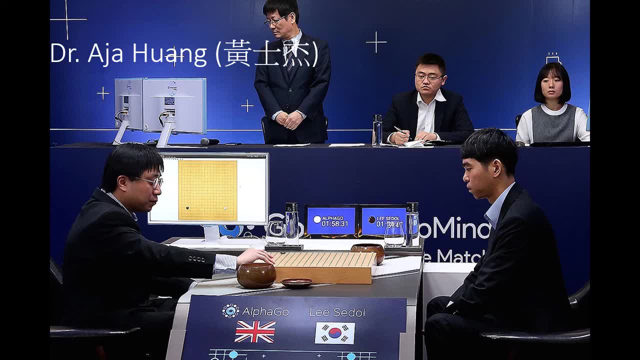 he studied PE in National Normal University. David Silver, the previous professor who told the best reinforcement online course and now working in DeepMind, finds the paper of Aja Huang and very impressive about his work of Go. so he invited Aja Huang to work in London and they published the paper of AlphaGo. 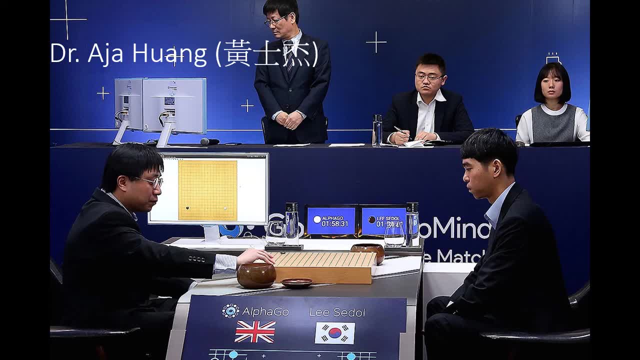 together. Aja Huang is the co-author of AlphaGo. Aja Huang is the co-author of AlphaGo. Aja Huang is the co-author of AlphaGo and he is the hand of AlphaGo when playing against Li Shudong, the BOTO of Aja Huang, when playing for AlphaGo. 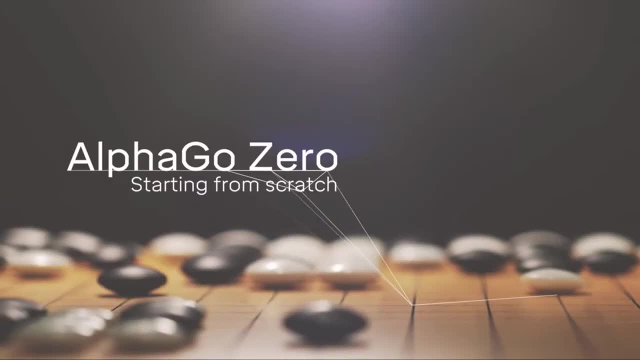 deep mind continued pushing the limit after beating the human world champion. In October 2017, DeepMind introduced AlphaGo Zero, which learns Go's new skill skill as typical Split players who are not that skilled in the game. which learns Go without reverting any human play records. 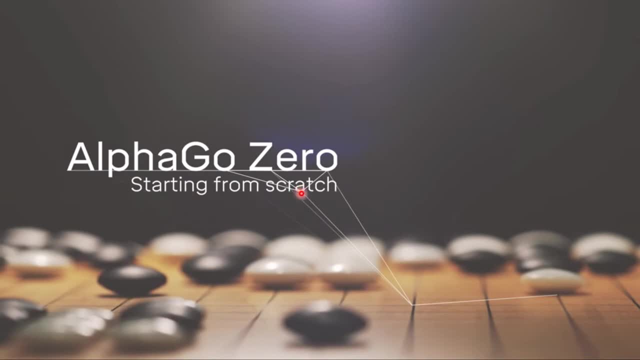 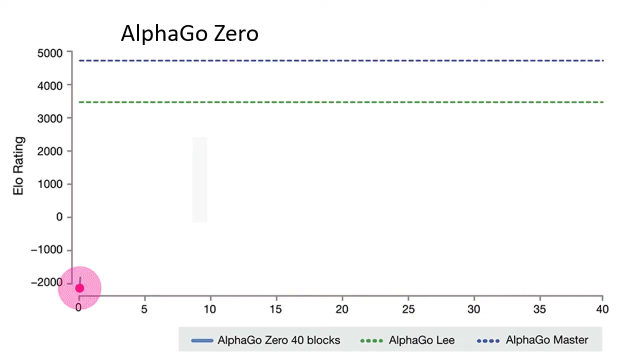 In other words, it's starting from scratch, So it's called AlphaGo Zero. Eventually, no one can understand the strategies behind the moves of AlphaGo Zero, which are beyond human comprehension. Let's see the learning progress of AlphaGo Zero. 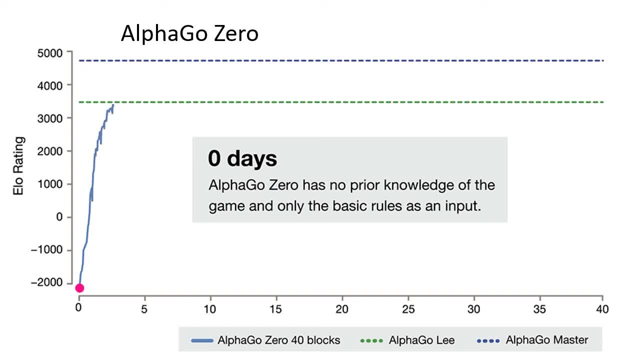 AlphaGo Zero has no prior knowledge of the game and only the basic rules as input. After 3 days, AlphaGo Zero surpassed the ability of AlphaGo League, the version that beat the champion Li Xudong in 2016.. After 21 days, AlphaGo reached the level of AlphaGo Master. 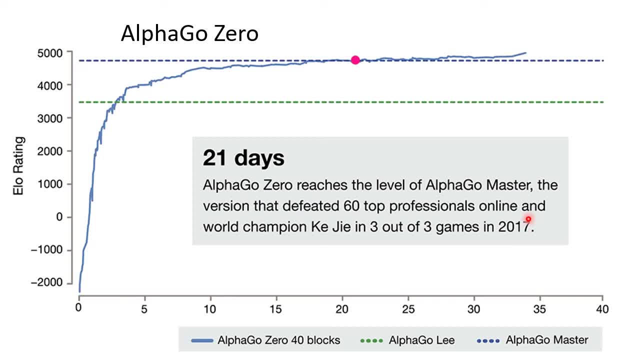 the version that defeated 60 top professional online and world champion Gejie in 3 out of 3 games in 2017.. After 40 days, AlphaGo Zero surpassed all other versions of AlphaGo and arguably becomes the best Go player in the world. 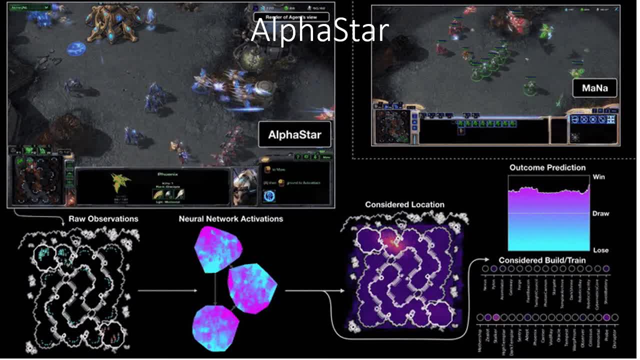 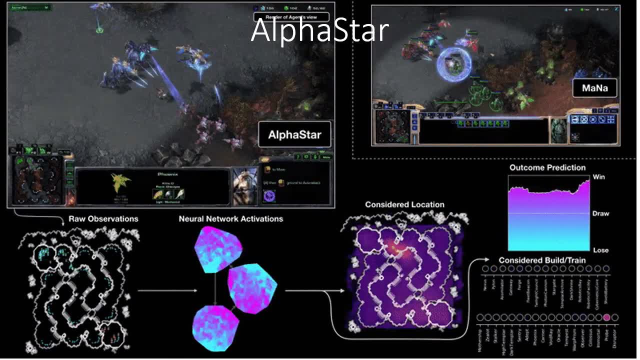 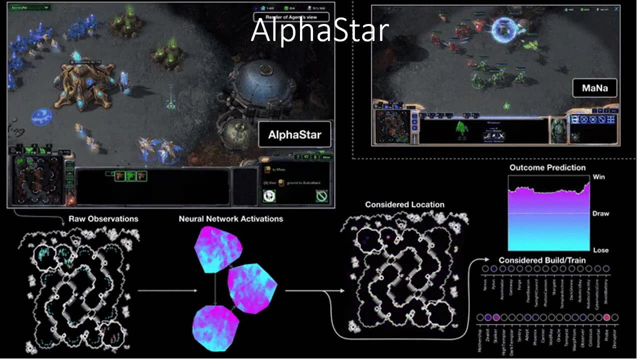 The latest work from DeepMind is Alpha Start, which learns to play the famous real-time strategy game, StarCraft. Although StarCraft is easier to play than Go for most people like me, it is partially observable again and hard for reinforcement learning In the game. 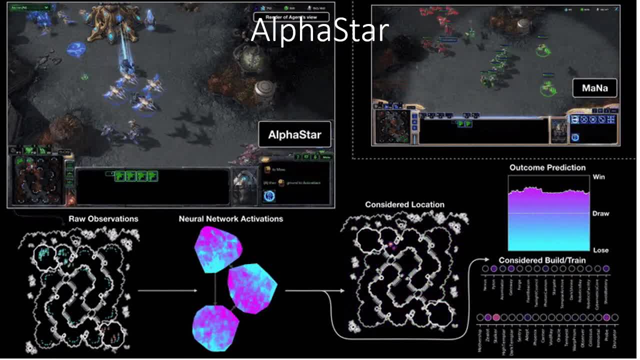 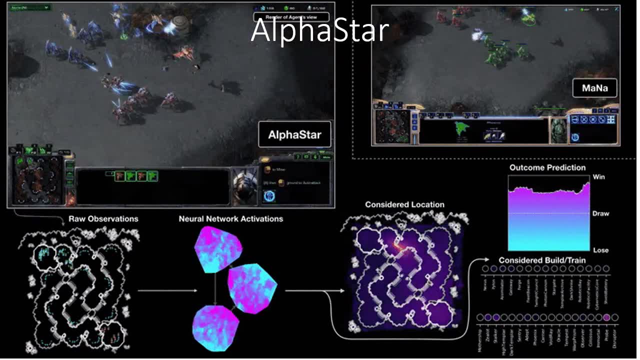 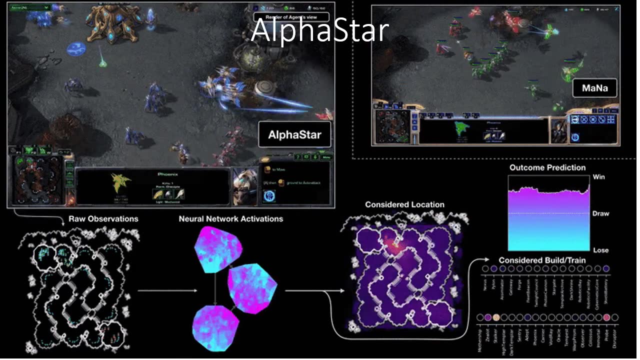 at the beginning of the game, the map is covered with war fog and each player can only see the neighborhood of his own troops. On the contrary, Go is a fully observable game that all components' moves can be viewed. Therefore, StarCraft is actually more difficult than Go. 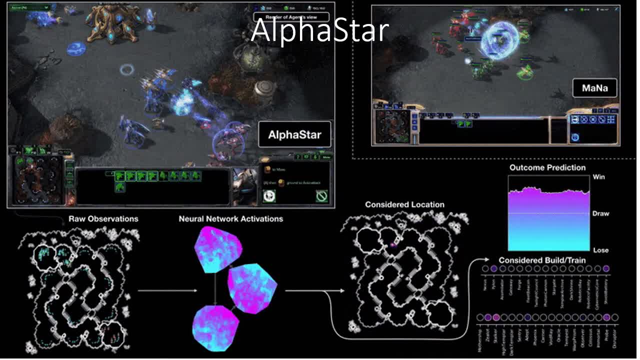 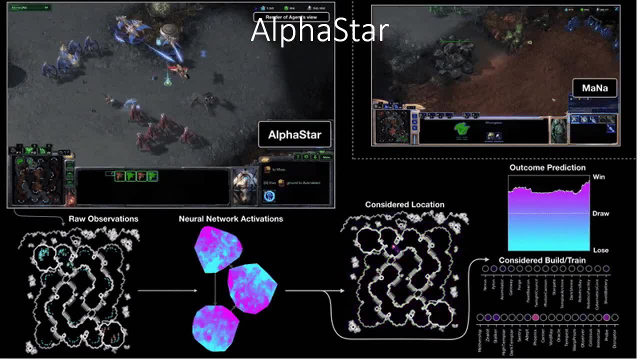 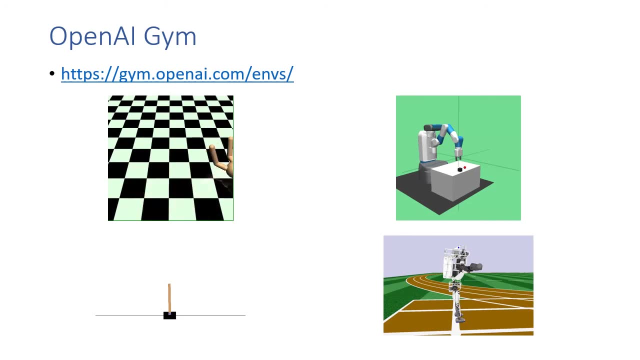 After 1 or 2 years of AlphaGo Zero, DeepMind managed to meet AlphaGo Star, which also beat the human master. To learn in reinforcement learning, we first need to have a good environment. Fortunately, the OpenAI has created many environments for us. 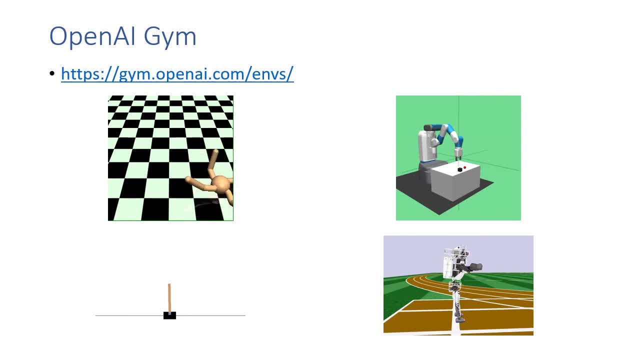 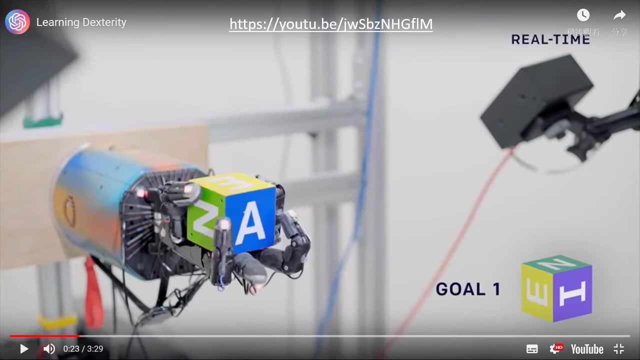 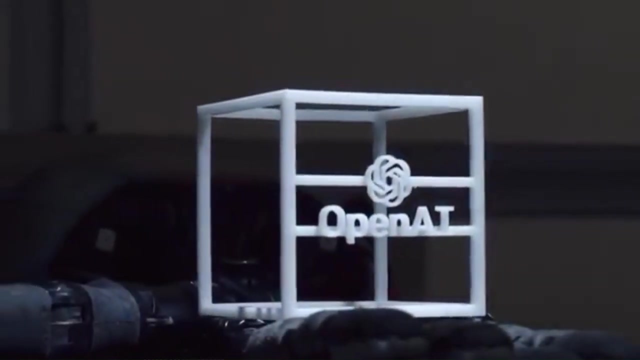 The OpenAI Gym is the most popular reinforcement learning benchmark. for many researchers, We will use OpenAI Gym for our homework and tutorials. Let's explore both environments for the first time. Please stay tuned. The OpenAI Gym is the most reliable and effective. 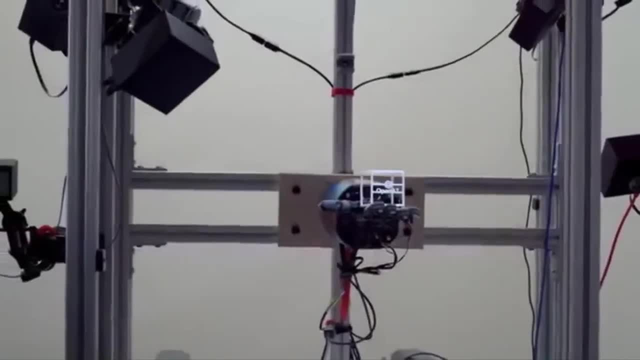 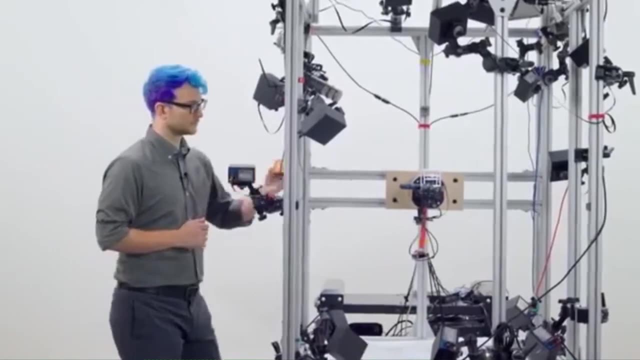 reinforcement learning platform for students. At this point, we used to do a high level of training. However, our students have only drawn 1 toös in the class and we have to shift to the other apartment. That was when we came to accept the instruction. 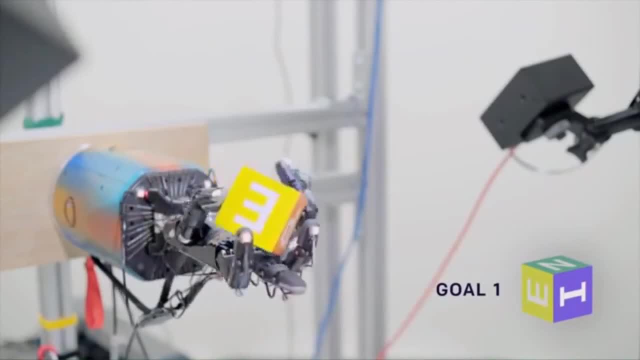 If you have any questions, please let us know in the comments. If you have any questions, please leave a comment. We're working on teaching robots to solve a wide variety of tasks without having to program them for any one specific task. Here our robot has learned to rotate a block into any orientation we'd like. 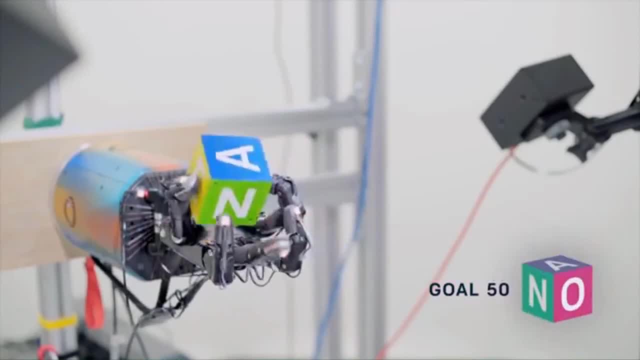 Once it succeeds at that, we give it a new goal, and so on. The system runs on a human-like robot hand and we use reinforcement learning and simulation to teach the robot how to solve tasks in the real world. To learn how to solve a task like this, we show it many different variations of the world. 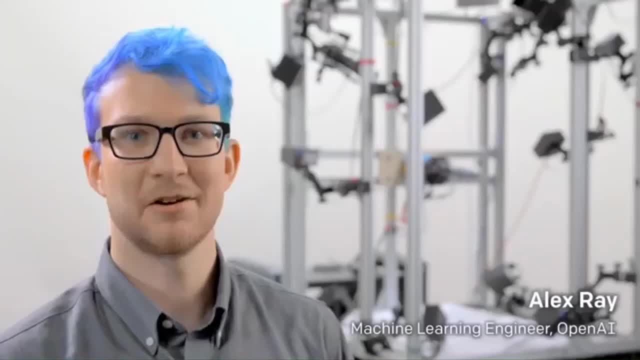 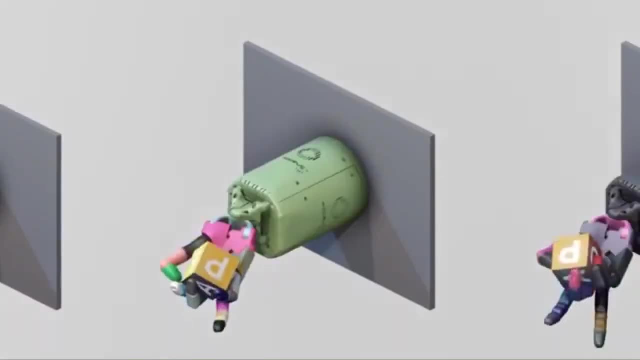 where the rules are slightly different every time. This is a technique called domain randomization and it affects, for example, the color of the cube and of the background. However, we take this technique beyond just how the environment looks. We also randomize aspects like how fast the hand can move, how heavy the block is and 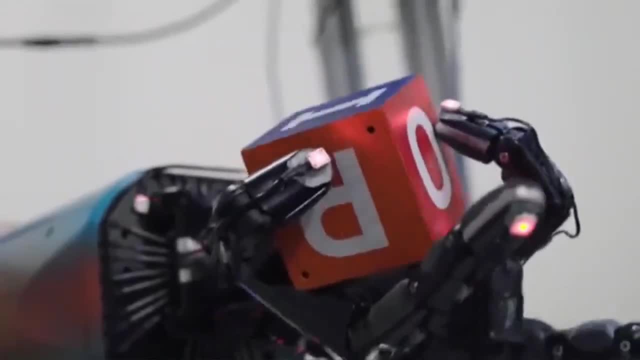 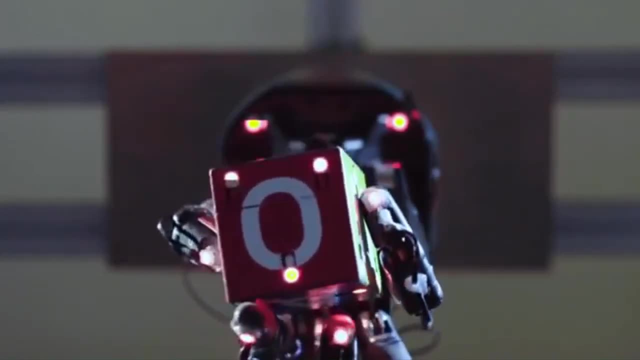 the friction between the block and the hand. Our learning algorithm sees all of these different worlds, and this lets it learn a way of manipulating the block that is very robust, Robust enough so that, eventually, we can accomplish the same task in the real world. 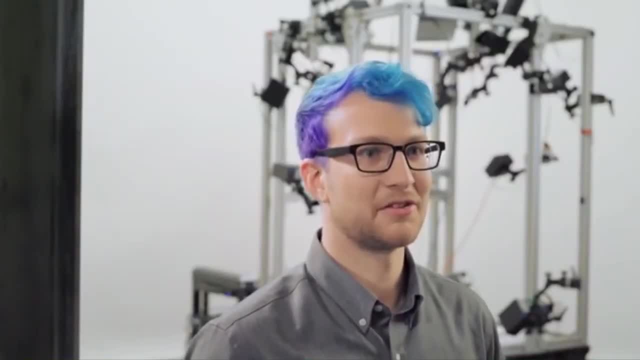 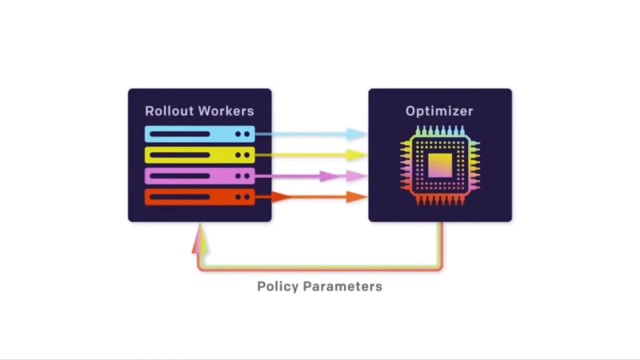 To simulate all of these possible variants of the environment, we've built a system that runs the training processes in the cloud on thousands of machines. It's called Rapid and we've used the same system before to solve complex video games. First rollout workers collect experience from many different variations of the environment. 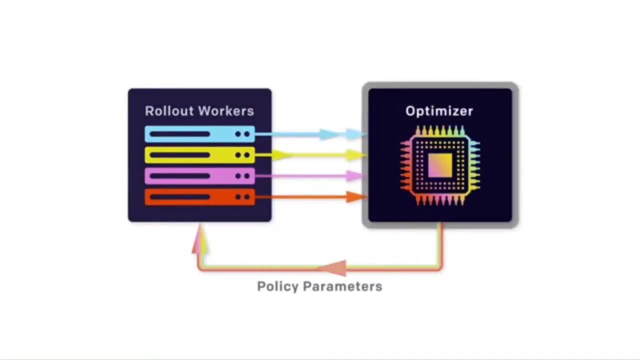 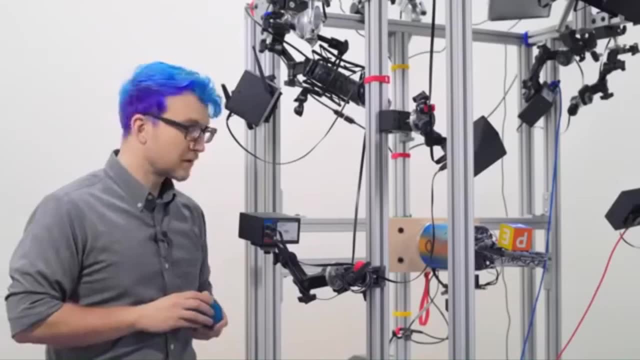 They send this experience data to the optimizer. The optimizer uses it to improve the parameters of the model controlling the robot. Finally, updated parameters make their way back to the rollout workers to complete the cycle. One thing that's very interesting to us is how general this system is. 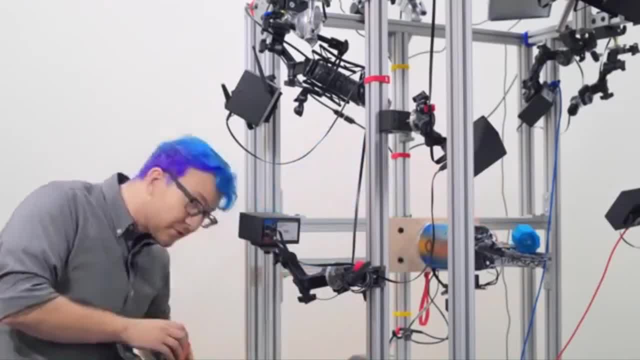 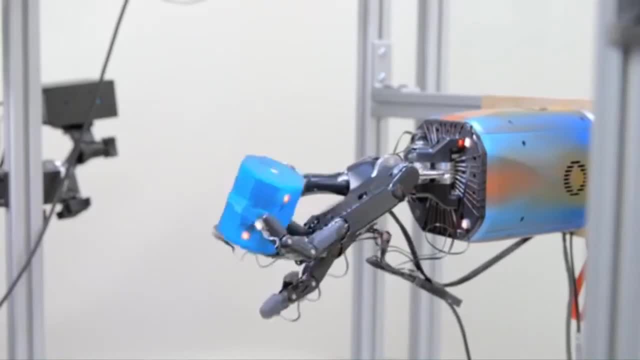 Not only can it rotate blocks, but it can perform tasks with other shapes as well. If you wanted to write a controller for this task, the old-fashioned way, you'd sit down and write out: exactly if I'm in this position, move this finger in this direction. if I'm.